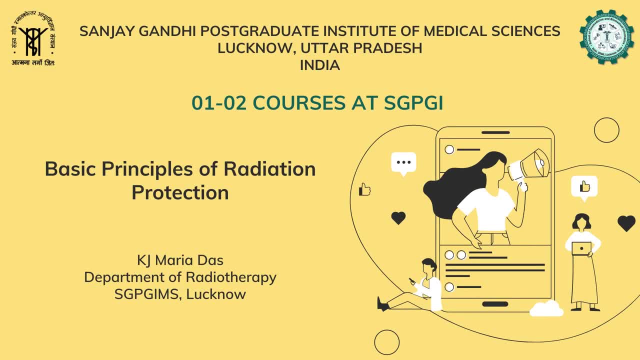 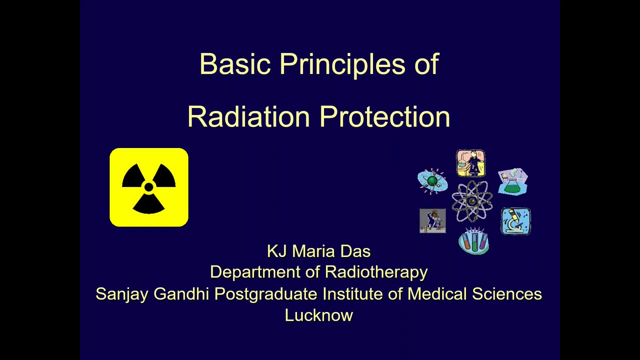 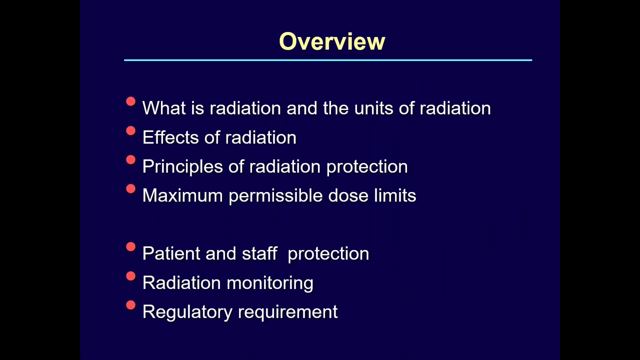 So I would be talking about the basic principles of radiation safety. Okay, so we know there are various. always, safety is a very important aspect, and when it comes to radiation safety, since there are many disciplines who are not aware of radiation safety, and so we thought 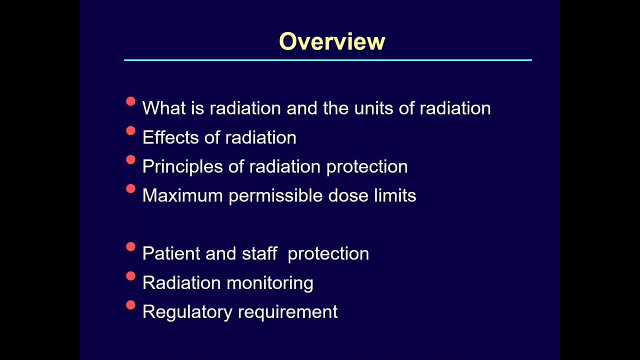 radiation safety should be made aware to all the people. So with this I thought I'll give you a brief overview about radiation. What is radiation? the units generally used and we know radiation effects. it is useful. at the same time, we have to have regulations and documentations about. 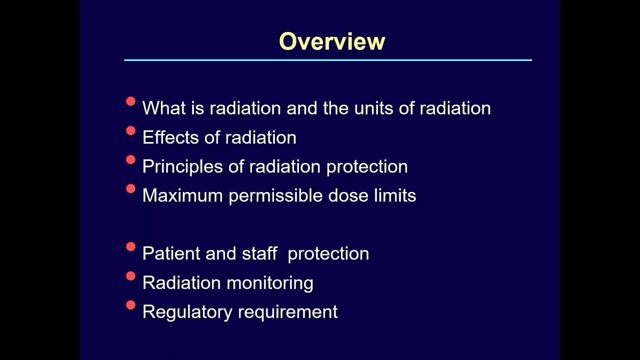 respecting the threshold doses for a safe radiation practice in a medical organization. It's not only confined to medical, it's also for industries also where we use radiation for the purpose of metal testing and other things. So I would be talking about the principles of radiation safety, the permissible dose limits as radiation workers and public. 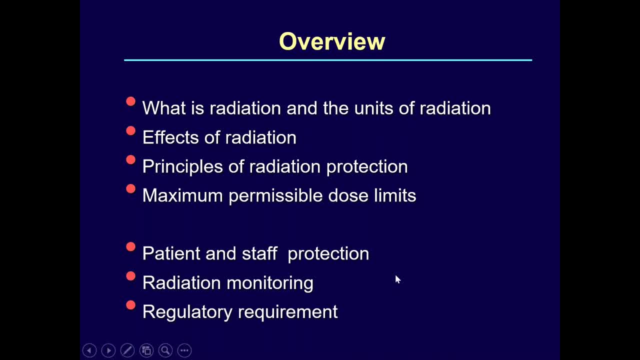 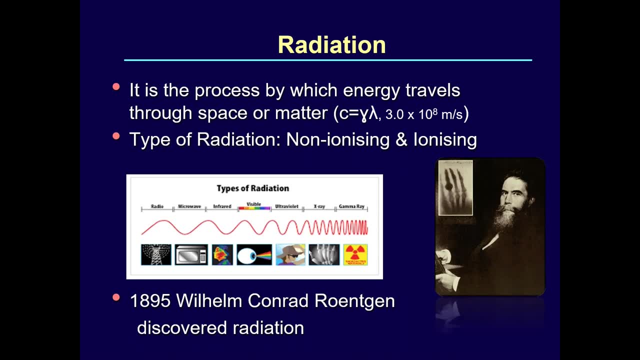 what we are entitled about, and we will talk about how the radiation is monitored in a medical environment and what are the regulatory aspects. So when we first come to the thing talking about radiation, what we always remember is control. William Rongen, He discovered the. this particular to you, okay. 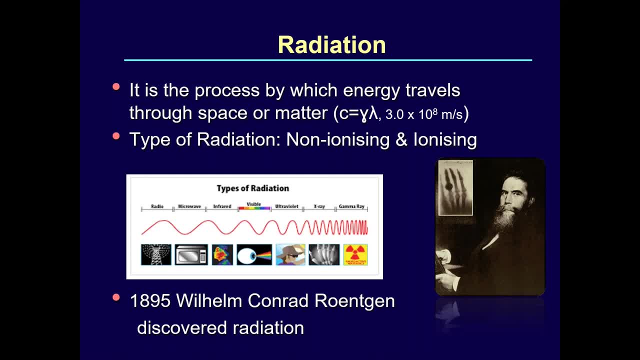 He just saw that invisible radiation and called this x-rays, and very soon he demonstrated that we can use x-rays to order for investigations to see a broken bone or a lung case for a pneumonia are a mammogram, without cut opening the patient. So that invention became a very normal one, and he was awarded the Nobel Prize in 1968.. You must regard information and information, have to care about condition and medical sett tr grading no matter what. But even with artificialGschas, behold, we could also see cases that can sound to cancer: lung cancerMUSE AirlinesasCardiac infection. Cool, what is the effect of so called an X-rays here? No matter what you write, next thingkanji. 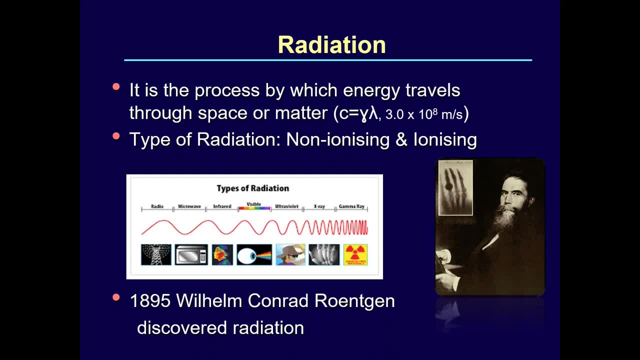 So when we talk radiation, all radiations of electromagnetic radiation, like light waves and everything, have a common principle, which is they all travel with the same velocity of light, which is 3 into 10 to the power, 8 meter per second. C. the velocity of light. C is equal to mu- lambda. mu is the frequency and lambda is the wavelength. 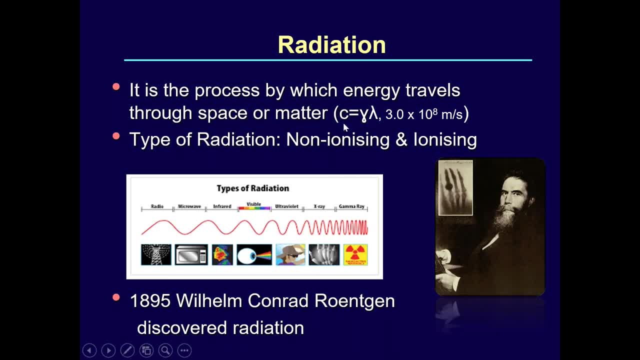 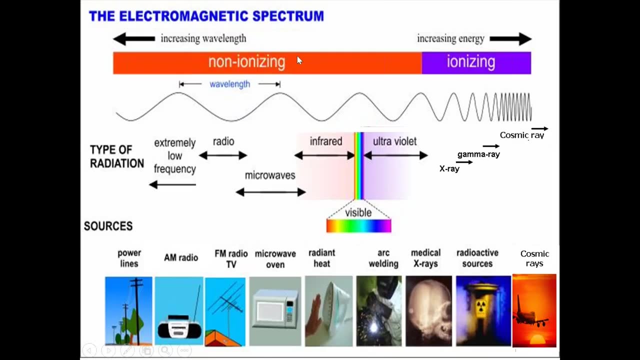 So as since we know the velocity is constant, the wavelength and the frequency will be inversely proportional: If the wavelength is high, the frequency has to be lower, if the frequency is high, the wavelength will be lower. So I will explain in the next one, like, if you look into this thing, the electromagnetic 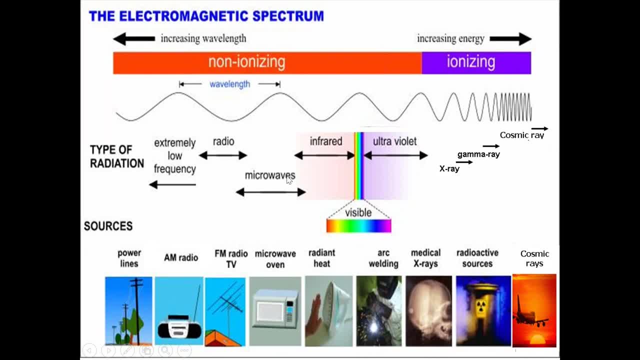 spectrum covers from radio waves to microwaves, infrared ultraviolet, So they cover the infrared ultraviolet, So up to ultraviolet Ultraviolet radiation. these things are classified as non-ionizing radiation and these non-ionizing radiations are used in power lines: radio microwave and everything. 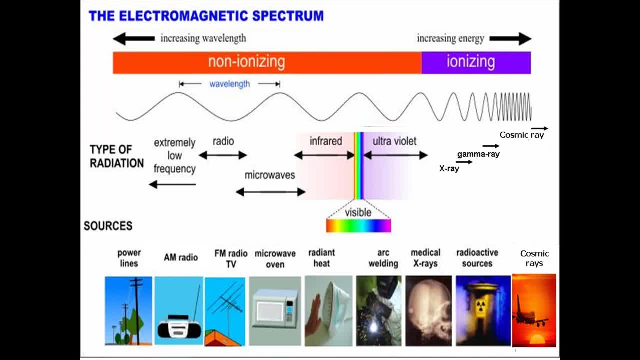 So although safety is important here, it's not that conscious like ionizing radiation, because the moment we come beyond the ultraviolet, the x-rays, gamma radiation and the cosmic radiation, they have the ability to ionize radiation, which could be harmful and certainly to be monitored well. 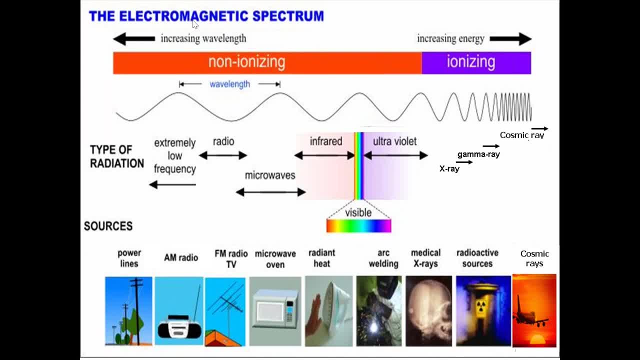 So now, if you see When the light waves and all the wavelength is quite larger. So as we go on in the spectrum towards the ionizing radiation, the wavelength decreases and the frequency increases. As frequency increases, the energy of the radiation increases and since the energy is higher, it. 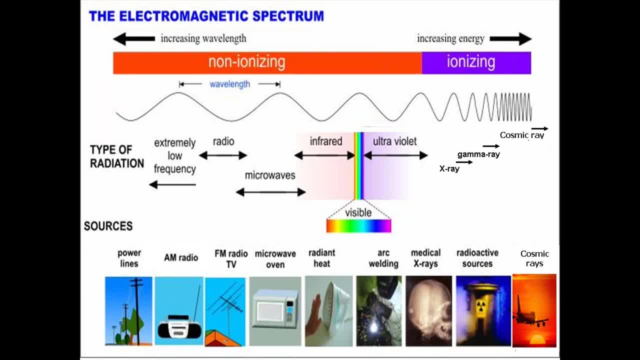 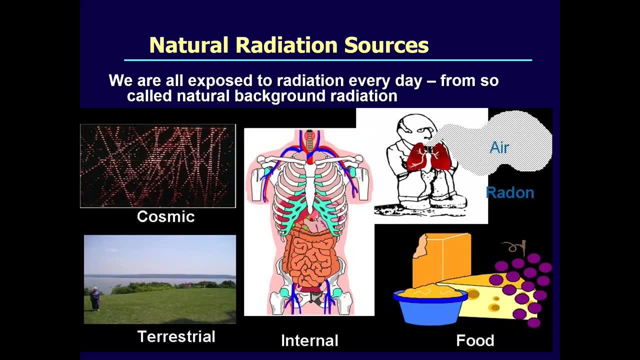 has the capability to knock out the electron and ionize, and it can also change the DNA structure, which can provide a lot of catastrophic effect. So now let us ask: Okay, So what was this question? Can we get rid of the radiation? If we look into the aspect, there is always natural radiation resources like potassium. 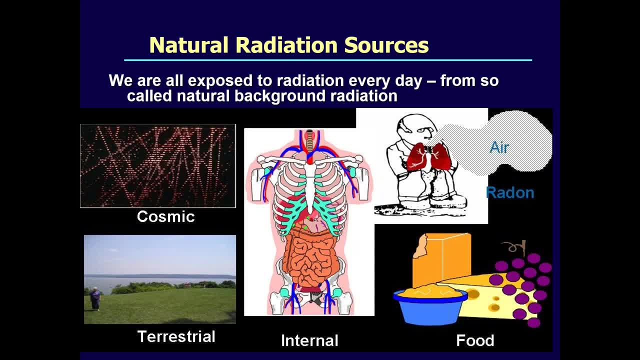 and many other isotopes, which is embedded in the rocks and in the living organism, by which we always have some amount of background radiation, and one of the major source of background radiation is the cosmic radiation, which is beyond the terrestrial and the atmospheric layer is a protective barrier for us. 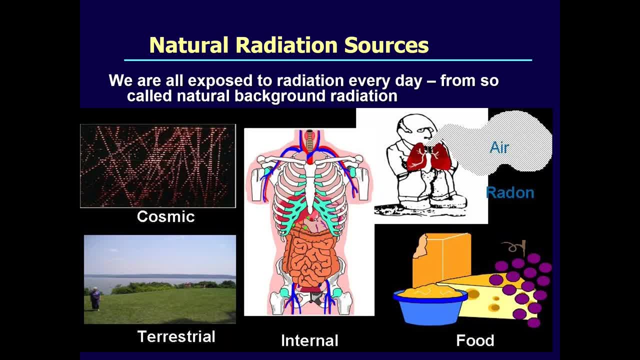 And since the atomic, The atmosphere is not having a uniform density, We have a variation in this cosmic radiations plus, because of the uranium, which has a very, very off life of radiation, which is in the billion and million years- uranium and thorium, There is a radium, again, isotope, which has 1600 years of off life, which has a counter. 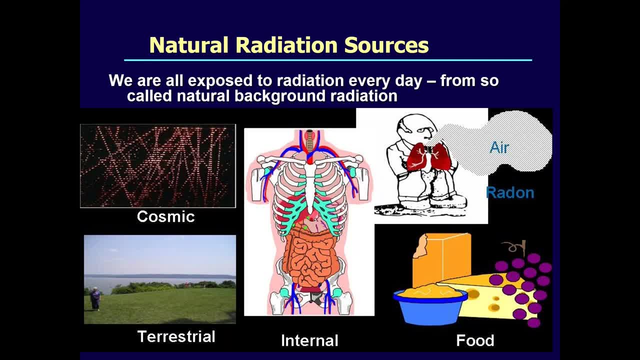 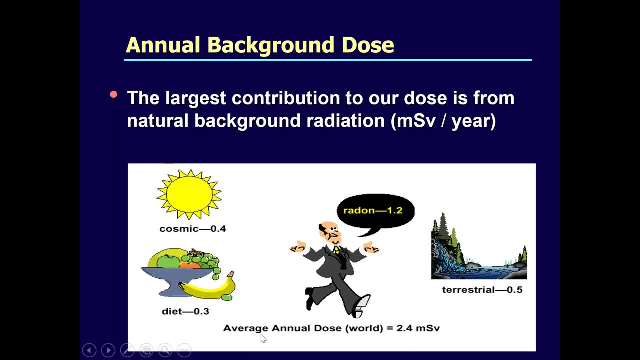 product which can come into a radon gas. So these things invariably form some amount of background radiation in the food what we consume or on the water that we intake. So this amount of radiation almost has been documented by the global organization, as the average annual dose is 2.4 millisievert. 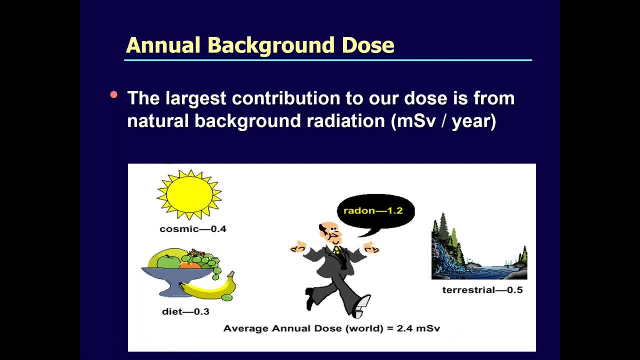 I will come to this units a little later, but please remember this: for radiation safety, we call them in terms of millisievert, Okay, and when we talk 2.4 millisievert, this is what is the background radiation contribution for average. So you could see from the cosmic radiation for the diet what we inhale, or the air what 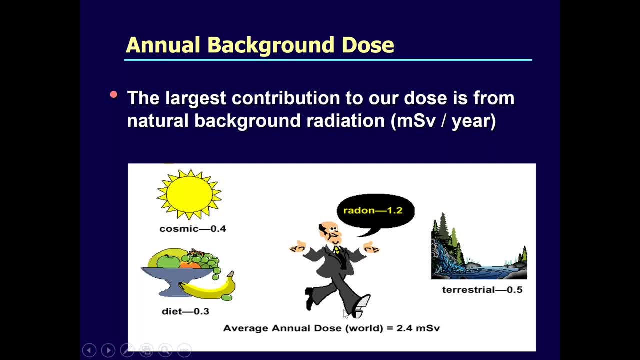 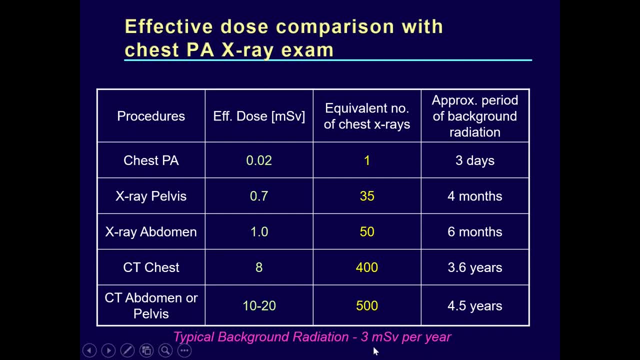 we use or from the terrestrial radiation. all to put together gives a 2.4 millisievert per year on average. So if you assume that 2.4 is the millisievert per year and this table is summating, giving a information about you, assume that 3 millisievert per year is the background radiation. 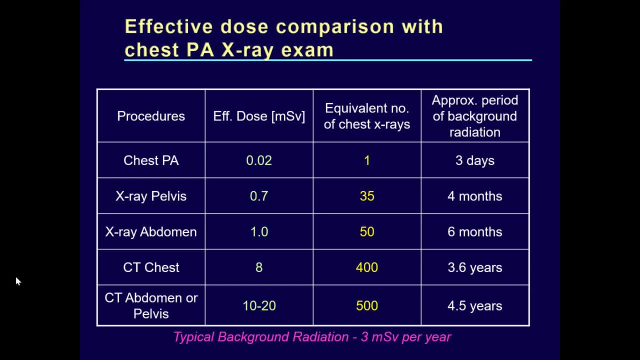 When we do X-ray investigations, Especially planar investigations like the chest X-ray or the pelvis X-ray. when we do, what kind of a dose do we accumulate? Is it substantial? If you look into the thing, we have 3 milli here. it is only 0.02. that means a chest X-ray. 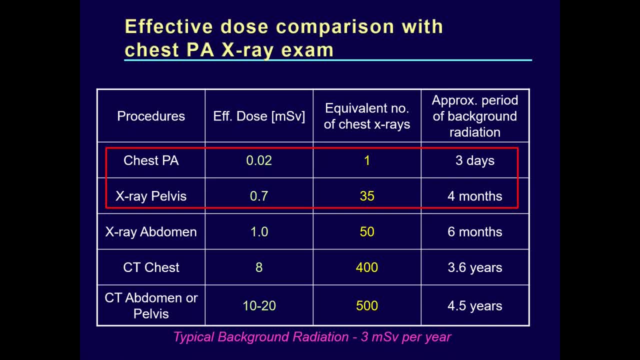 is the one which consumes the lowest radiation exposure. Why, compared to pelvis, chest consumes lower? because chest is composed of lung. lung doesn't attenuate that much, That much like a tissue or a bone. So in order to take a chest X-ray, you have to give the least MA and KV. 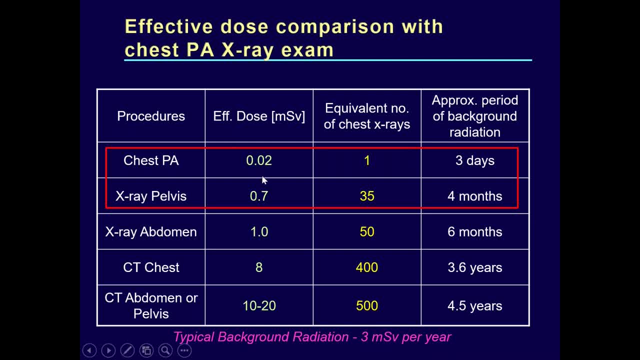 So if the effective dose by a chest radiation is only 0.02 millisievert and if you take this as one unit, it is just like a three days of background radiation. That means doing one chest X-ray. the patient is at a not at all at a risk because he is. 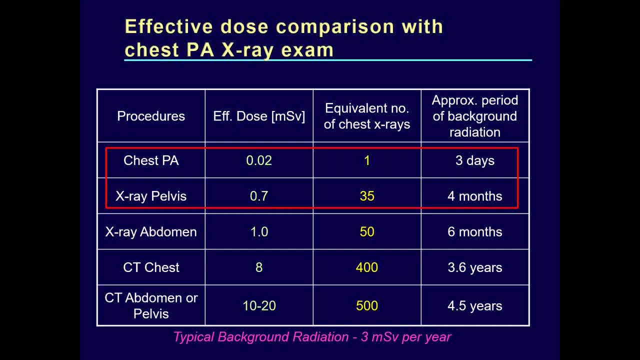 just getting three days of a background radiation. Inevitably the background radiation Is not that harmful because we are all are living in that and we are not produce any considerable effect on that. So the moment from the chest X-ray you come to a pelvis or abdomen, it goes from that to 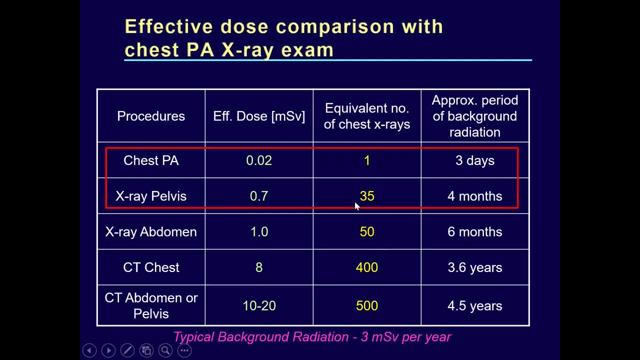 0.7 or one, which means it goes 35 to 40 percent, 40 times higher. So even in planar X-ray, chest X-ray is the simplest and the X-ray which consumes the lowest radiation dose, So it can be frequently used for diagnosis. 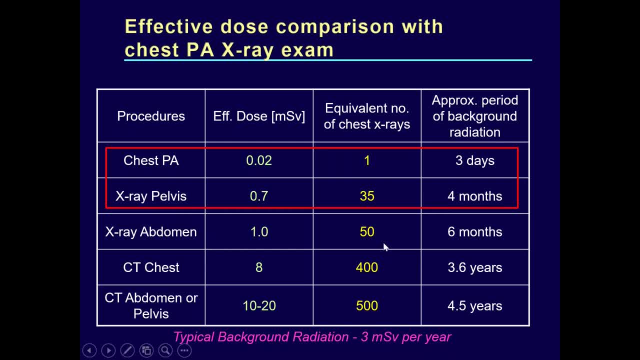 And then the pelvis X-ray is the simplest And the X-ray which consumes the lowest radiation dose. The pelvis and abdomen consumes about 40 percent of the dose of a chest X-ray. Now, the moment you come to volumetric imaging, like a CT of the chest or CT of the abdomen. 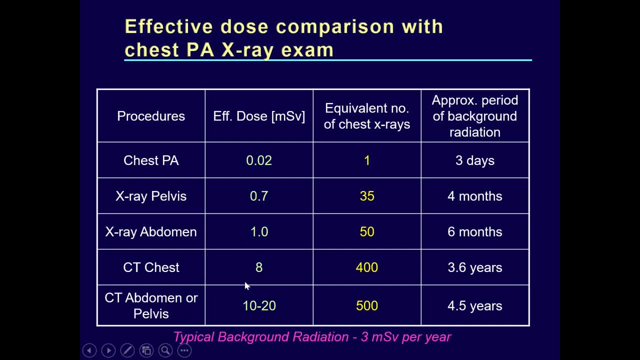 it further increases by tenfold the radiation, like 8 millisievert, 10 to 20 millisieverts, which means it is like 3.6 times the average dose of the background radiation. Is that clear? So, in order to say, the chest radiation gets a larger dose compared to a background radiation. 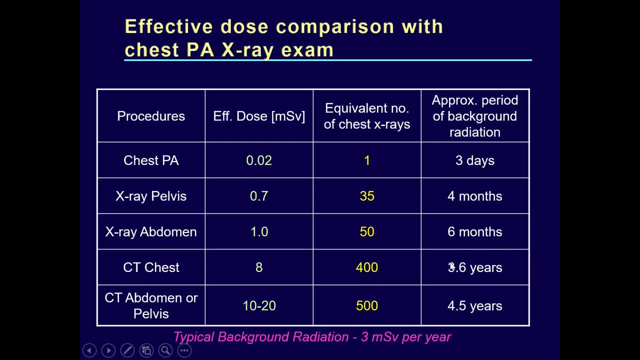 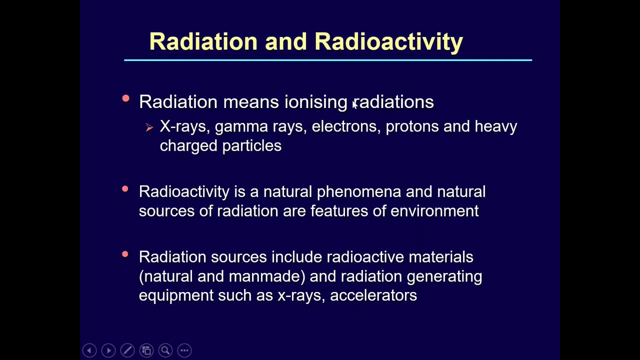 like 3.6 times the background radiation, what you could have consumed per year. So now coming to the thing talking about what is radiation and radioactivity. Radiation means we talk about here in this lecture ionizing radiations which could be coming out from a X-ray machines like a X-ray C arm or a linear accelerator like that, or 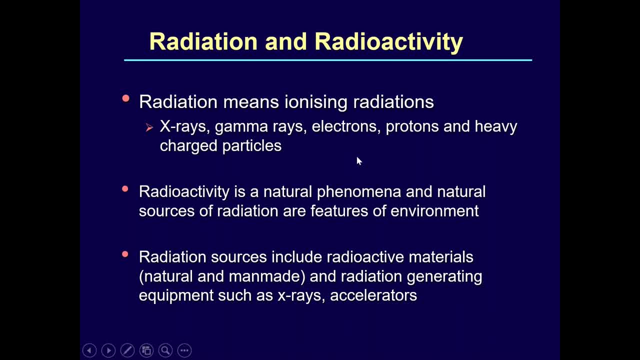 gamma radiation, Which comes from a radioactive isotopes or electrons and beta, trans, protons and heavy charged particles are also used for research purpose as well as therapeutic purposes. So radioactivity is a natural phenomena which we have already learned in many of our textbooks that it radioactivity has two kinds. 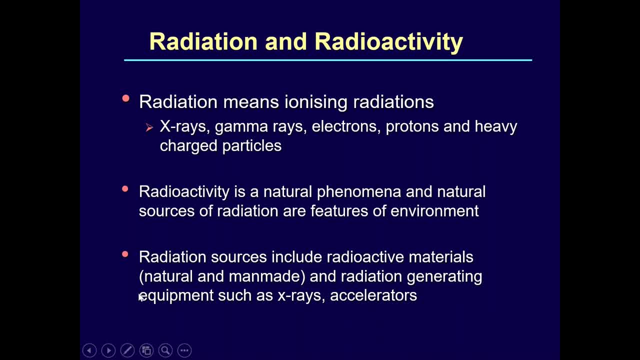 One is man-made and another one natural resources. Natural radioactive materials generally have a very long off life and we have to live with that Now. in the case of background radiation, when you compare it from Kerala to Kashmir, the Kerala part has a larger background radiation because of the rocks are rich in thorium content. 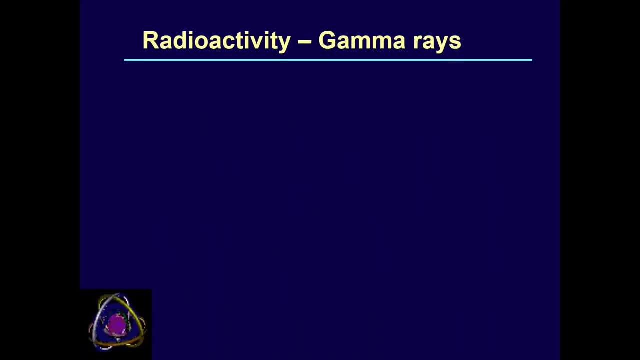 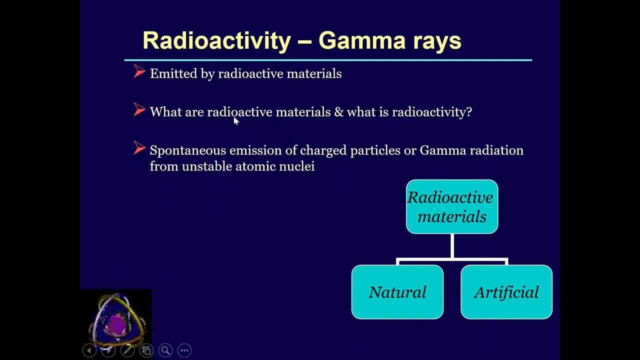 compared to the other parts of India. Coming to radioactivity, we have to remember one thing: since it is a spontaneous emission, it can. it spontaneously emits till it comes to a stable stage. during that it produces either gamma, beta or alpha, So it can come to stable stage. 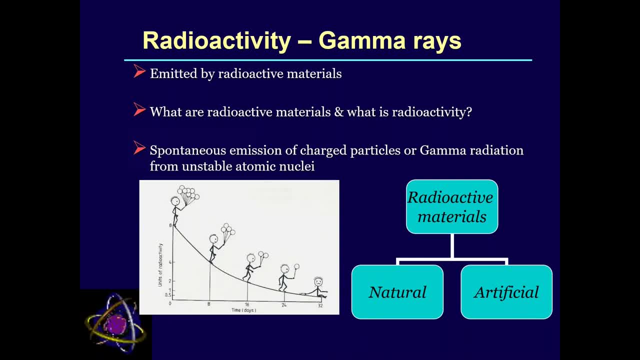 and it comes to a stable place. by reaching this, and if you assume that in this graph, if you assume a radioisotope just having a half-life of eight days, what is half-life? half-life means the original activity to be reduced off of its initial activity, the time period taken for the original activity to be 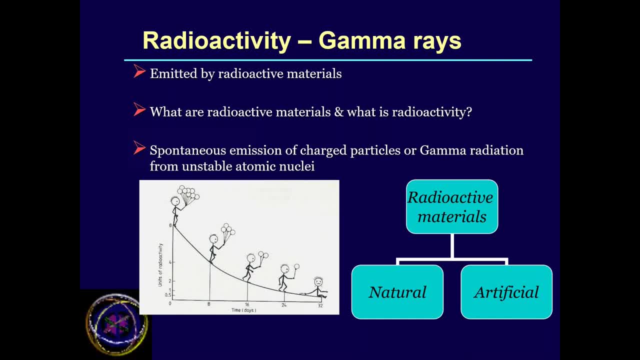 reduced to arts off of the initial incident activity. so if you assume here that this was having 16 balloons and in order to reduce it to four of its activity it took eight days. so next half-life for it will reduce to two in another eight days, which is 16 days. next, from two to one in another eight, which 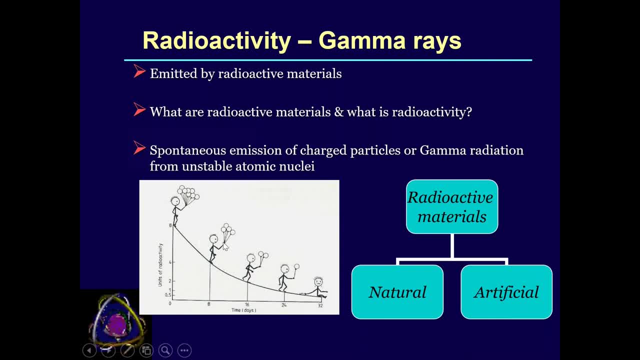 is 24, and so when you come up to four half-lives- one, two, three, four- the radiation is considered to be negligibly insignificant in terms of a radiation damage. but this doesn't happen in the case of radiation damage. but this doesn't happen in the case of. 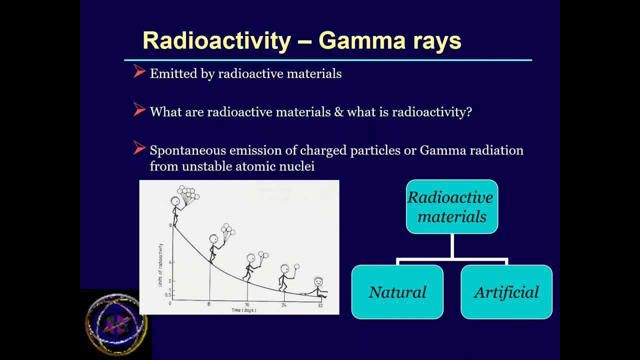 hold it through. true, if the activity is very large, if it is a small activity which is used in nuclear medicine, we can assume that after four half-lives we can dispose them. but if it is in a therapeutic department like this, other activities, or in million curies, so that activity will be still sufficiently. 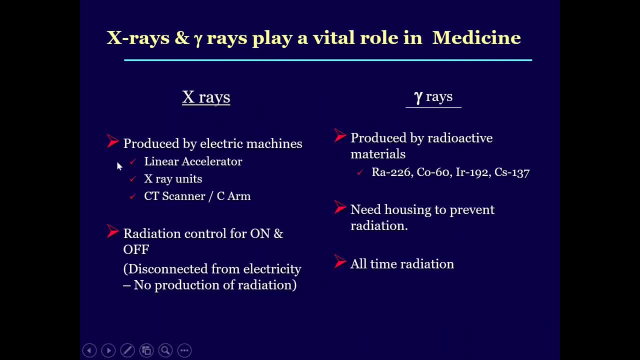 large enough. so coming to X and gamma rays play a vital role in medicine. the x-rays are produced in linear accelerators, C arm CT scanners and, except for us, the advantage of x-rays is that it is having a radiation control, on or off. that means when we are giving a radiation, the 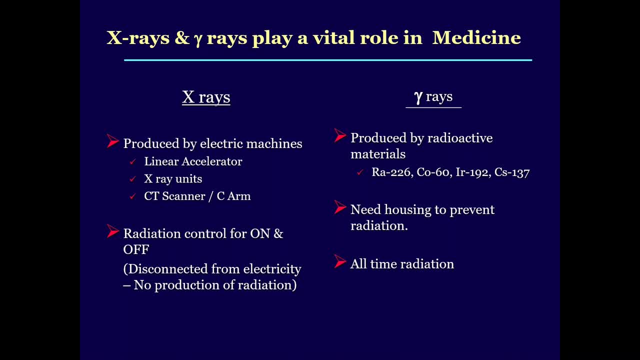 patient is also getting a radiation. there is a scatter radiation and beyond the control console and the vicinity where the public is walking they will get some amount of extra background radiation. but the moment the x-ray unit or the control console is switched off there is no radiation. that means the 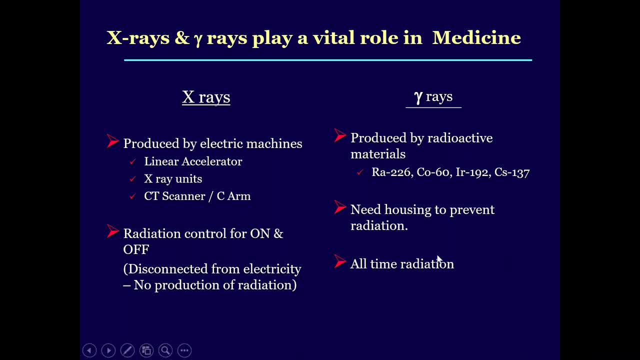 radiation is safe. when it comes to the means, the patient is in the right position. we have radioactive isotopes like a gamma-rays, which either used in gamma rays or beta us. we have isotopes like radium-226 or cobalt or iridium, which is used for industrial. 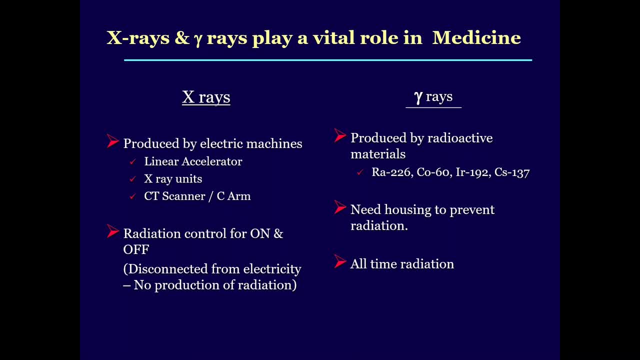 brachytherapy. they always need to be housed in a big protective housing carrier and from that carrier they remotely come for a switch on position and switch off position. that means even when the radiation in the off position advantage is the radioactive isotopes used for the purpose of diagnosis or therapy in the medicine. 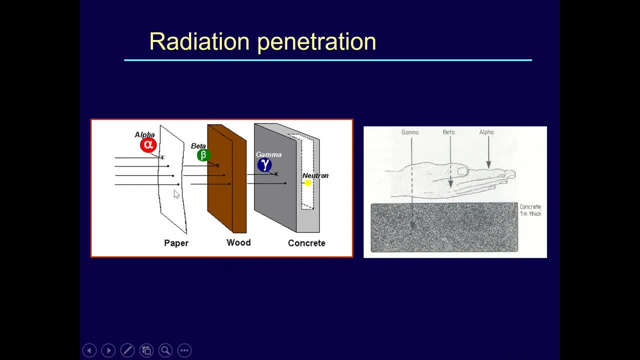 and just this slide to illustrate again. when we talk about different types of radiation- alpha, beta or gamma- we have to remember that alpha particle is heavy charged particles which can very well attenuated in a thin piece of paper. when it comes to beta or electron particles, a 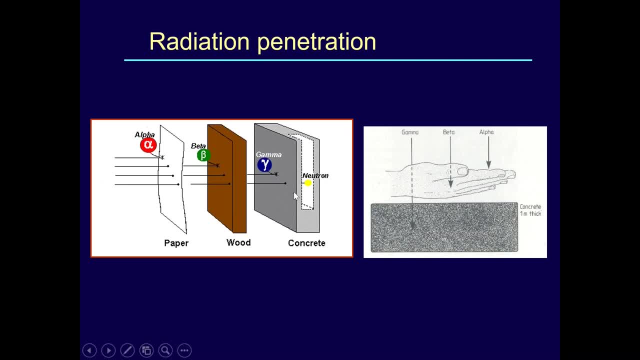 wood or a perspex material will be a good enough material to attenuate, whereas a gamma or x-rays can even pass on through any concrete materials and high density x-rays. they can interact with high density materials in the concrete, with steels or something to produce neutrons. 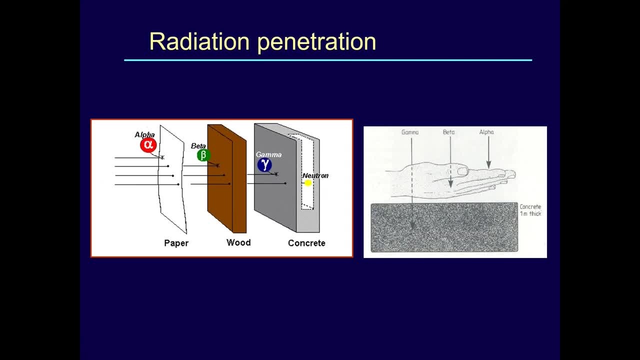 so when you have a very high charged x-ray missions you do have neutron barriers to control the background radiation so that the people who work beyond that radiation environment, because radiotherapy or nuclear medicine and radiology forms a part of the hospital. so the radiation safety takes into consideration, though the public works, the adjacent areas, the 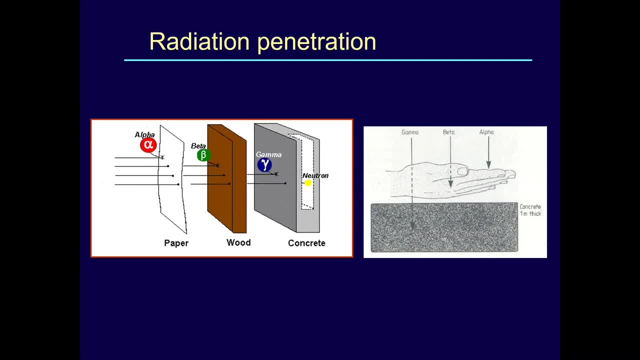 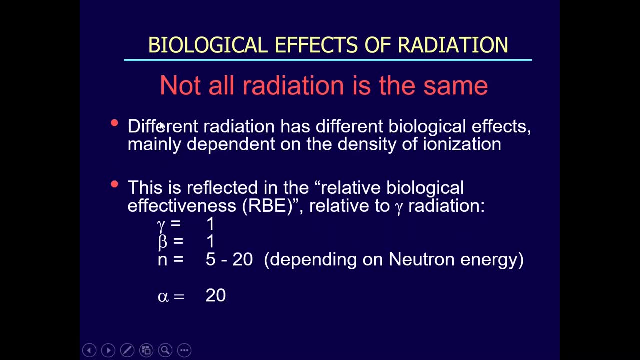 patient, public or the professional radiation medical fraternity working nearby areas are safe. so when it comes to another question, sorry. so another thing is: does all the radiation, that intensity may vary but beyond that, for a same amount of intensity, does their biologic effect? effectiveness is the same. 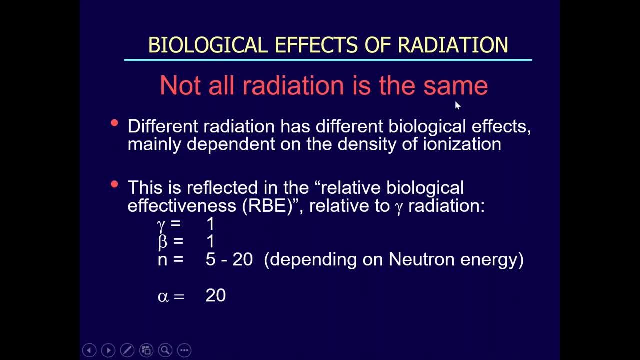 the answer is no. different radiation has different biological effects. mainly depends upon the density of ionizing radiation in one aspect, in the physics aspect, we call it let. linear energy transfer. that means in a cubic millimeter how many radiations can pass through. that is called as a let and in 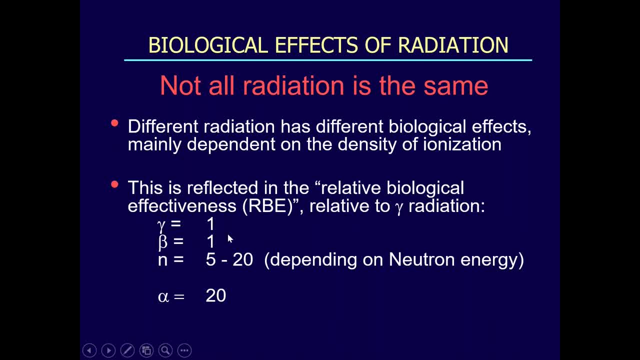 a biological term. we call it a biological equivalent, relative biological effectiveness, rbe. so this rbe will be changing with different type of radiation. so for x and gamma it is one. for beta, it where we use for neutron radiation, it can range from 5 to 20. for alpha it is 20.. that means what? 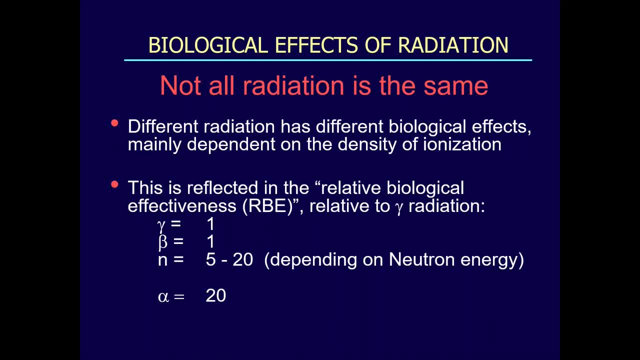 we have to keep in mind is that if a patient is getting a neutron therapy, their doses would be much less for the therapeutic and similarly, if you are getting a dose for by incident you have got some neutron contamination or something, the biological effect will be 5 to 20 times larger. 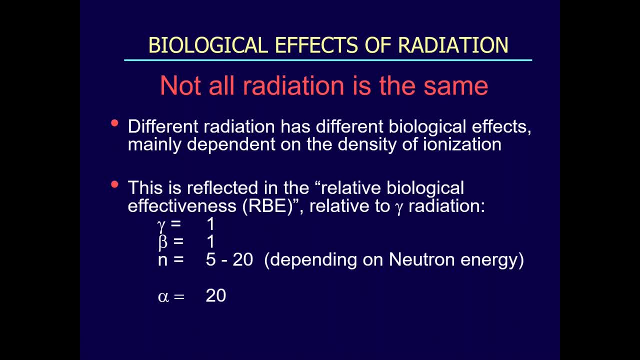 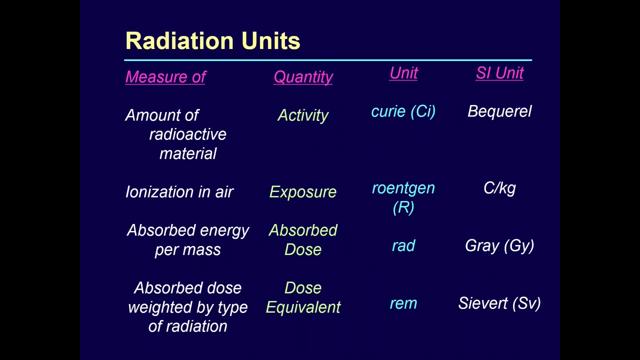 so for radiation safety, it is a very important aspect to see what kind of a radiation exposure a person has and what its biological equivalence would be in terms of to assess the hazard part. so since we are talking about radiation, we also remember some of the things when we talk, when we 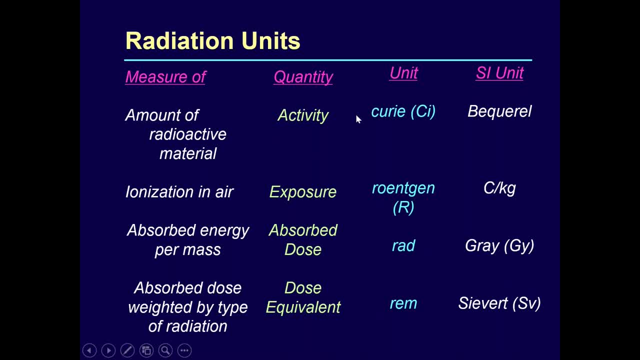 learnt about radioactivity, the madam mary curie. well, i discovered the radioactivity and on her name the unit curie was given. so curie is a unit which is used, and the si unit is vacuole- for radiation x-rays. we use wrong gen, ronkin ronjan, and the si unit is coulombs per kg for dosimetry purposes. 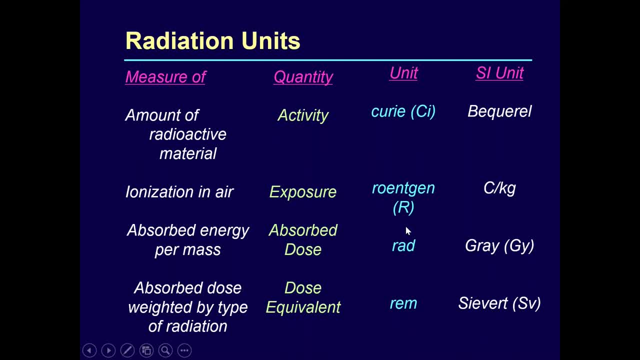 but this ronjan is an exposure radiation. that means from a x-ray certain radiationers are coming out and it is an exposure. but after exposure the absorption in the body will be different for bone tissue and lung. for lung it will be 0.4 times for tissue, if you assume it is 1 for bone it. 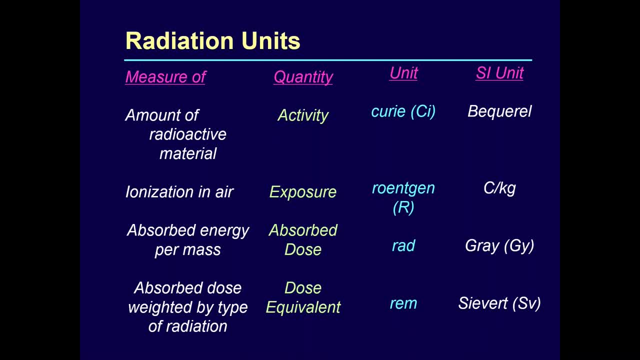 could be varied from 1.4 to 1.8 times attorney, which means the absorption done on bone would be larger. so we have another dose, which is called absorbdose, in the form of rad or gray used in the therapeutic purposes. now this is okay for practicing. when we come to radiation safety, we have another term, what is called dose? any rad, a dose of rad, an, not an interval during submission, are the two cases we have: a available dose of cheek or leucine, another term called²- too safe physics talk about- or non toxic term. what is called dose? each standard of radiation which is amplified in the target practice. so we have 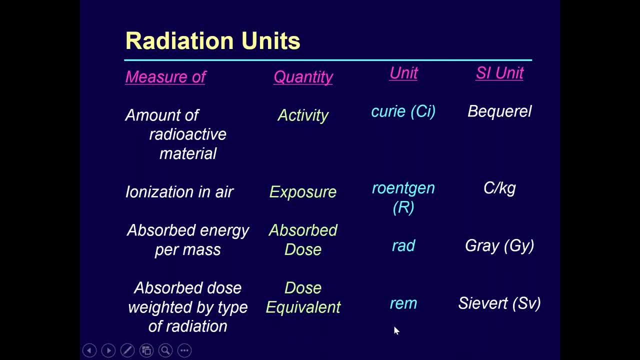 that to choose one of the two processes totally different where we are having ronkin and ronjan, are they which are the two strategies which are not certified as applied to reference to this dose equivalent, where we call it as a REM, which means rad equivalent met, and the SI unit is: 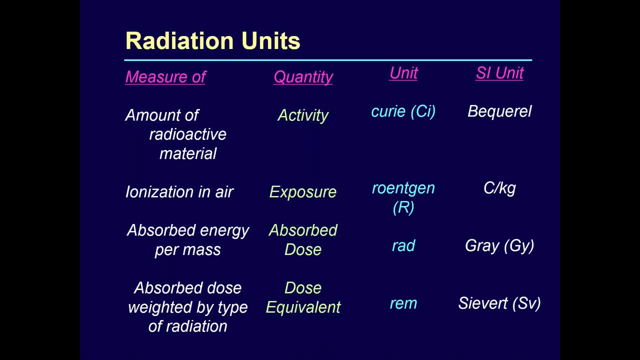 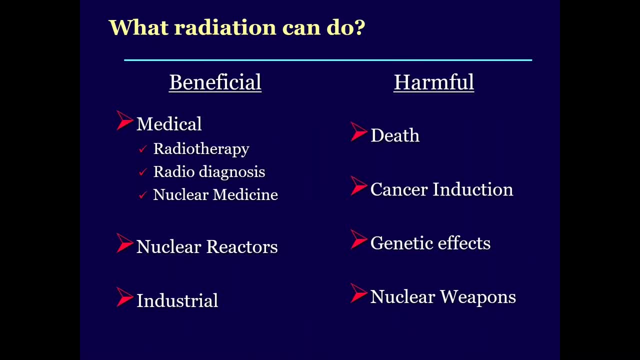 Sievert. You may remember that when I talked about the background radiation, I tell it is about 3 millisievert per year. So now what radiation can do? Radiation could be beneficial when we use in radiotherapy or radio diagnosis on nuclear medicine. It is also used in nuclear reactor to 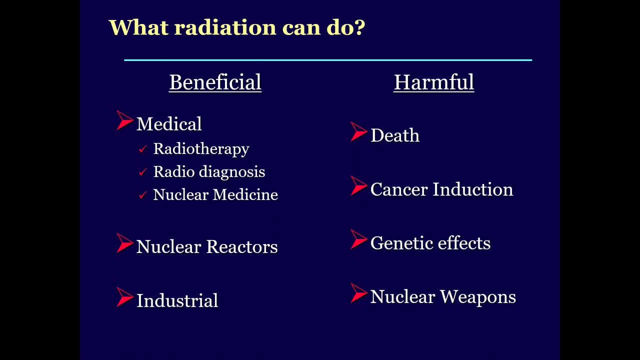 produce radioactive isotopes Industry also. it has been used to test materials for cracks and other things. but at the same time, if they are not being used properly- and there is a thing- huge amount of radiation can cause death. It can have cancer induction and long-term radiation. 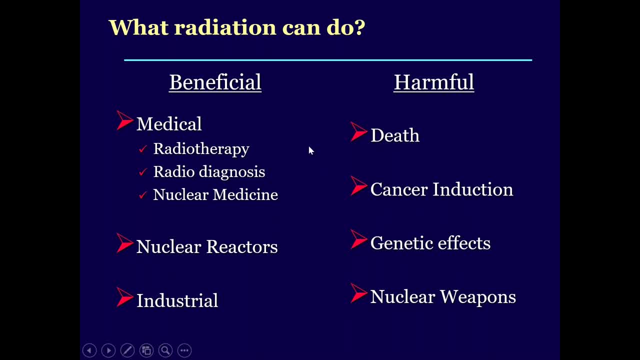 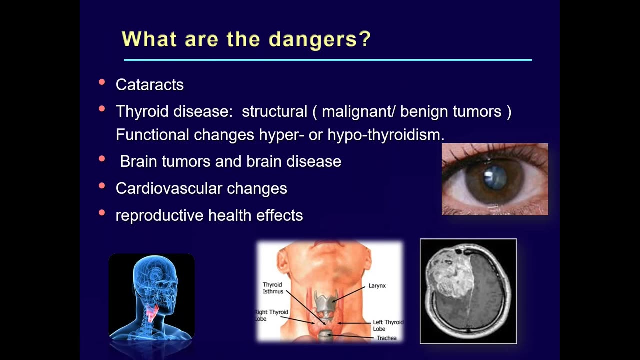 effect can be producing genetic effects, and nuclear weapons could be created from these radioactive isotopes as nuclear bombs. So is it dangerous? Yeah, radiation is dangerous If we don't monitor it and have a safe practice. if the doses are larger it can form cataract. it can have thyroid diseases, it can have functional changes, brain. 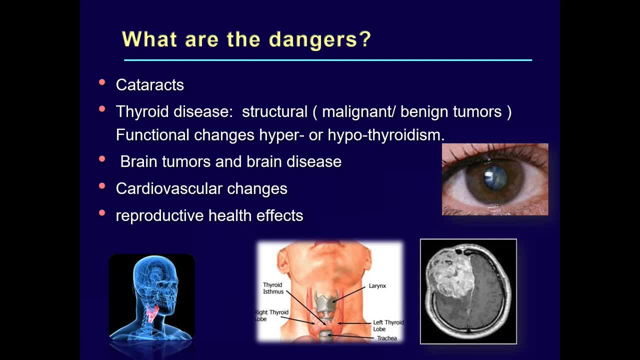 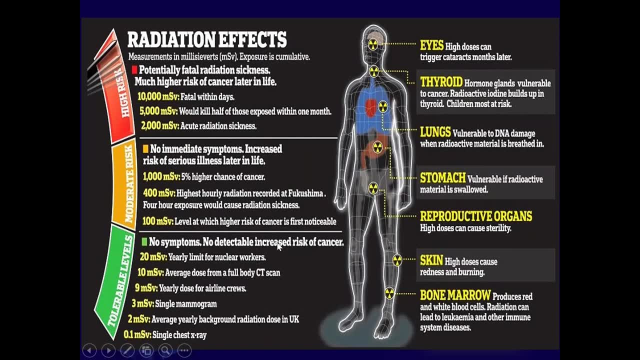 tumours, cardiovascular changes, reproductive health, So various things it could have. So now you look into this, this graph, this chart, which I generally like it, because here the green portion gives the radiation doses which are within the tolerable regions, Like if you look into people. 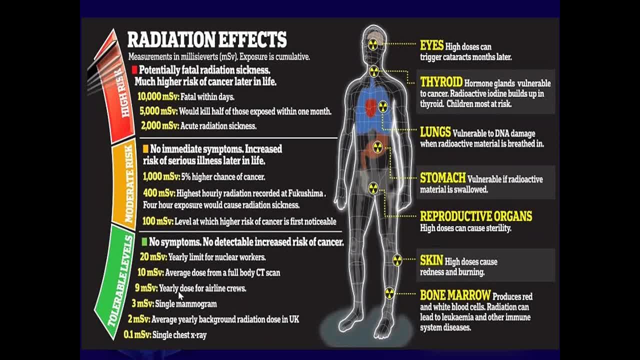 who are often flying on the aircrafts. Example: the pilot. By virtue of going above the atmospheric pressure, he always gets a larger amount of a background radiation like 9 millisievert per year. So and the cruise So even up to 20 millisievert. up to 20 millisievert, it has been. 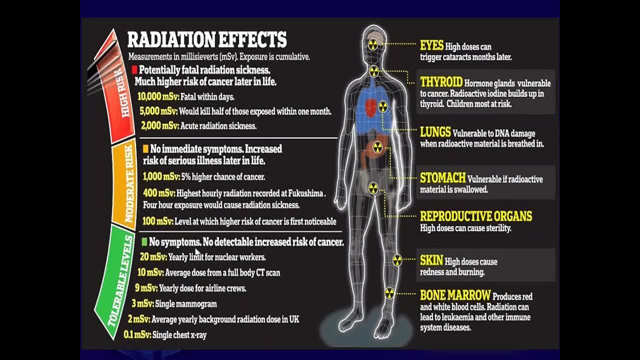 considered to be tolerable and there is no effect, which means even 1% also will not. no one will have a cataract or any other cancer induced disadvantage of a hair loss due to a dose up to 20 millisievert- Not even 1%. So from there, when you come to moderate amount of radiation doses, like in the 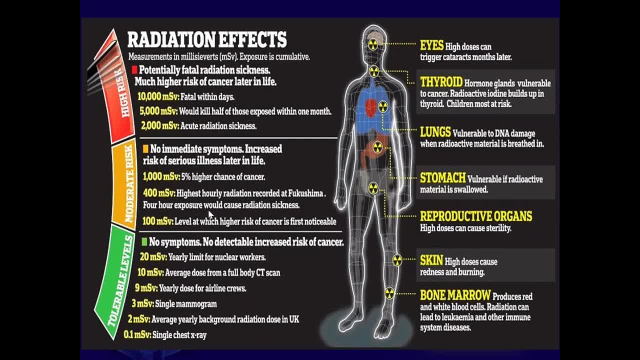 nuclear medicine or anywhere, even in radiotherapy. if there's a radiation source truck or some radioactive isotope has been removed by mistake by a vendor and given it to a scrap dealer and it got into the public or anything these radiations, then there's a possibility of having a radiation dose something. 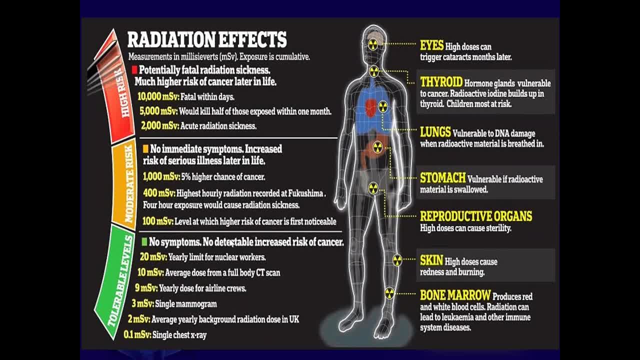 like this: 100 millisievert, 2000 millisievert, and here you can have some mild effects of intermediate effects at putting a little risk. but the doses beyond 200 millisievert, these kind of a doses we have seen in the Japanese radiation accident. 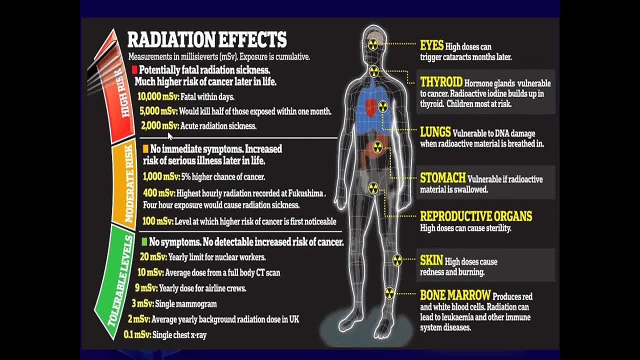 And those. history has taught us that these kind of a doses could lead to fetal fatal effects. like 10,000 will have a fatal effect and 5000, 2000 have really produced tremendous sickness to the patient: radiation, acute sicknesses And radiation by virtue- if it gets to a skin it could have a skin sperm burning if it gets. 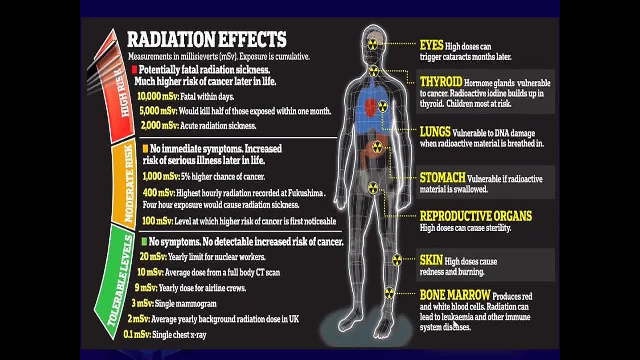 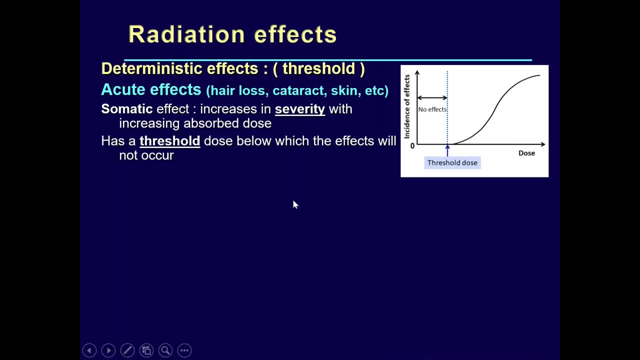 to the marrow, the cells will interact with the DNA and change the characteristics and it produces a reproductive way. So now we know the radiation effect. when radiation effect again, we can classify into two types of effects. one is deterministic effect. when we say deterministic effect it has a threshold. 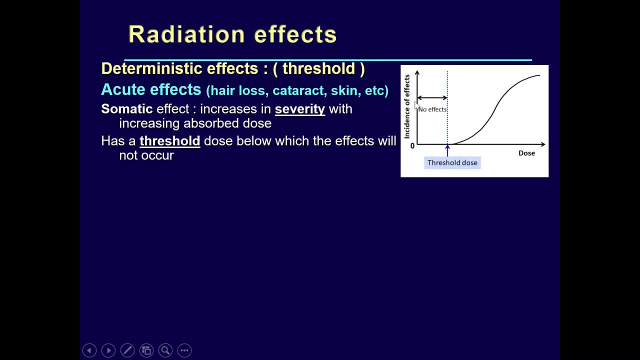 you see the curve: up to a particular value there is no effect and after that it forms a sigmoidal curve As a function of increase in dose. so the incident of the effect is in the y axis. the x axis is dose and as the dose increases the incident of the effect will form a sigmoidal curve. 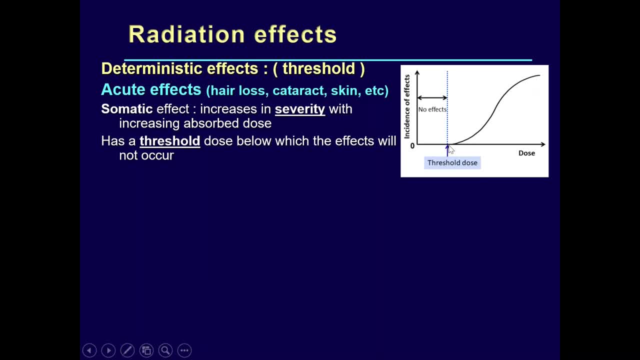 and this below the threshold dose, there is no effect. and even beyond this threshold dose also, it will be less than one percent of the persons may have such a kind of incidence. it's very less chance Still. But for the safety point we have to respect this threshold dose. so beyond this threshold, 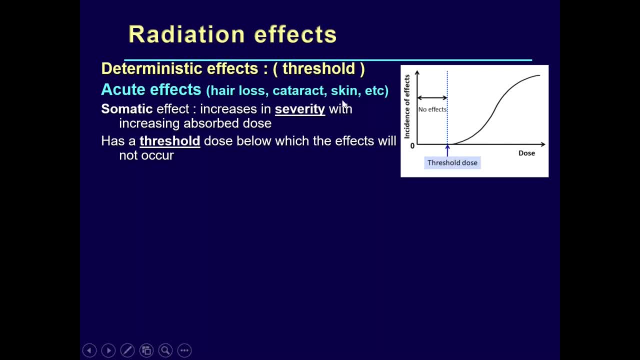 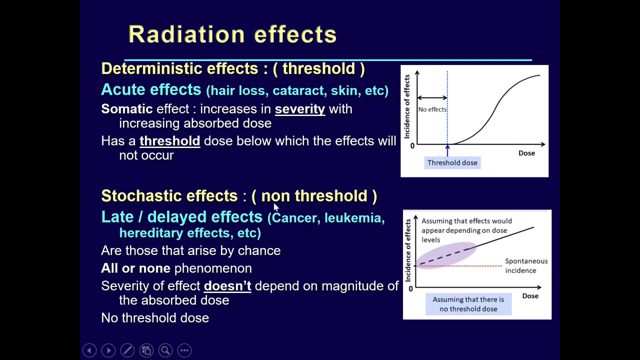 dose. if we to have, it can have a hair loss or cataract or a skin ban, and these are generally called a somatic effect, and this effect increases with the increase in dose. The other effect is stochastic effect. stochastic effect means it doesn't have a threshold. it 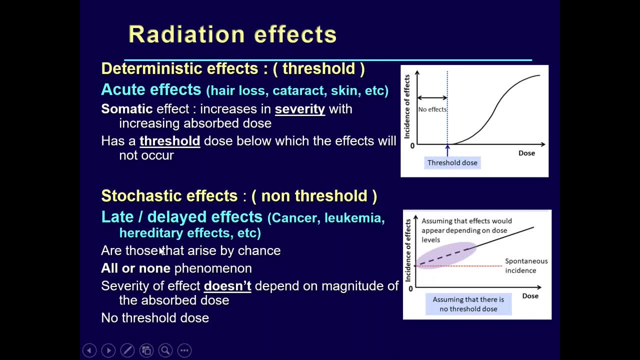 is linear and this can have late effects And In case of cancer, in secondary cancer induced or a leukemia or a hereditary like a breast cancer coming up to the second or the third generation, could be a effect of stochastic effect. Here either it happens or it doesn't happen. it doesn't have that like a, the effect doesn't. 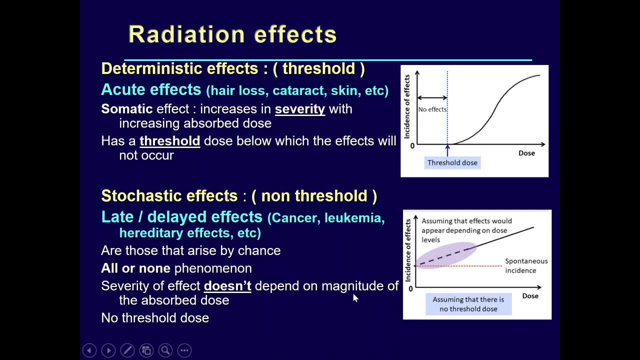 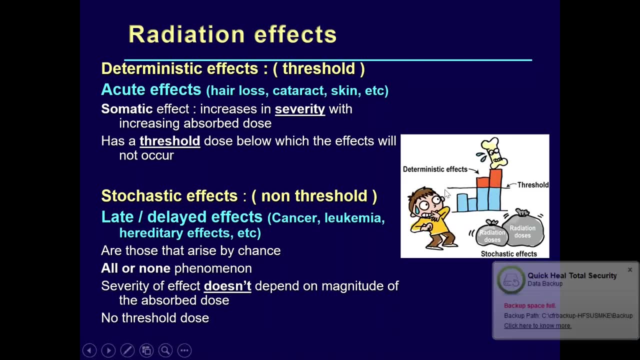 increase. the severity of the effect doesn't increase with the magnitude of the observed dose. Okay, So no threshold for stochastic effect. For Deterministic effect there is a threshold, since, like, if you see deterministic effect, we have to respect the threshold dose. then we are much safer when it comes to stochastic. 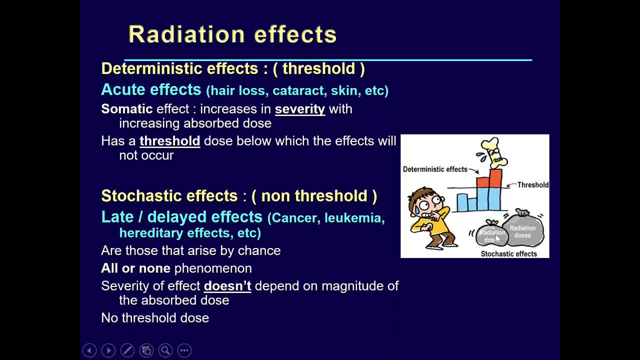 effect. there is no threshold dose. whether you do a small radiation dose package or a large radiation dose package, the probability of the effect could be, and it's not necessary that the larger dose person only will get the effect. the lower dose person also may get the effect. 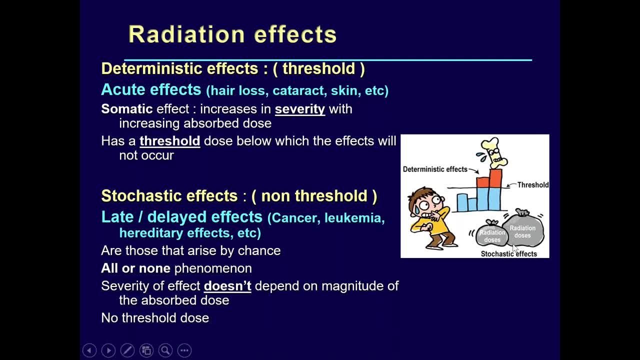 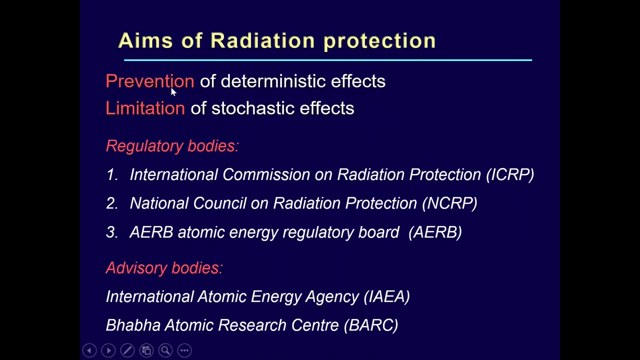 So this is a really a producing a big challenge. that means from this we can understand deterministic effect as a threshold by which we can try to control. but stochastic effect we cannot control. So the radiation safety principle taught us that we should prevent the deterministic effect by respecting the threshold, the stochastic effect. we cannot do that way, so we have to. 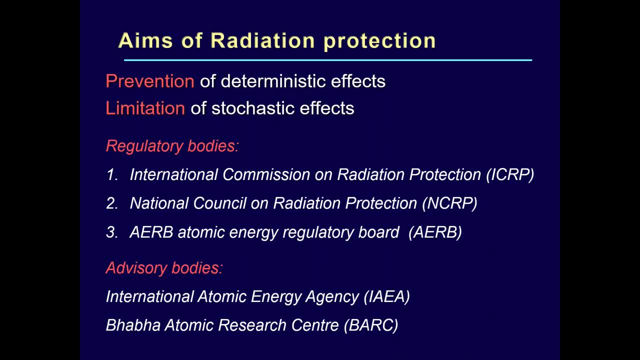 do limitation And Apply as low as possible. we have to have the minimum radiation possible. So this is where radiation safety is much different from the other safety. okay, a fire safety or a biotic safety is different from radiation safety, because no radiation is useful. 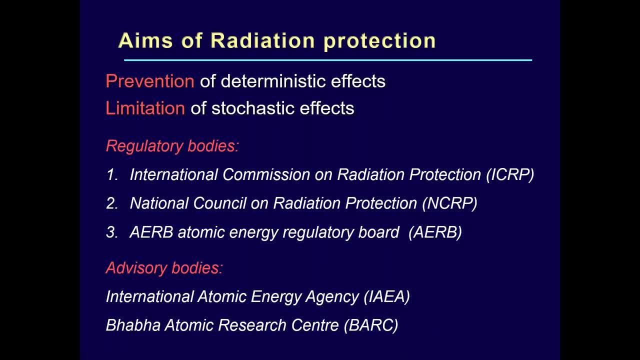 So we have to see as low as radiation possible for public as public, and understand the deterministic effect and respect the threshold dose. for that we have regulatory bodies like international commission of radiation protection, national council of radiation protection, and for India we follow the atomic energy regulatory board. so who is the regulatory body in India for? 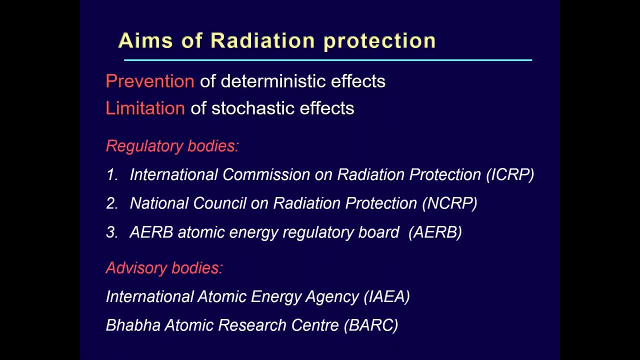 giving us licenses and whom all the medical institutions have to obtain license and have the inventories and have to monitor the radiation safety of patients as well as the area and the medical facility and report to them. and they keep controlling us. And now there are two more advisory bodies. one is international atomic energy agency. 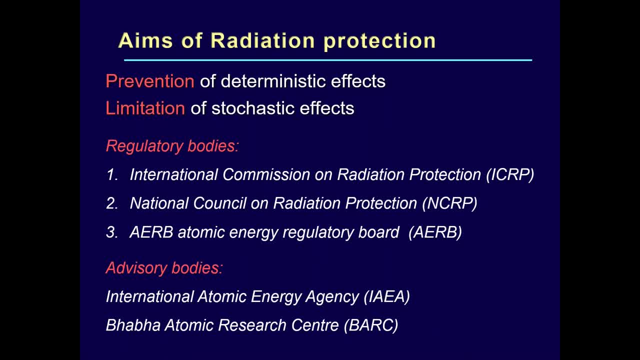 So they do more research on radiation and its biological effect and suggest for documents for radiation protection and like that, in India we have baba atomic research center, where they do have facility for making artificial radioactive isotopes as well as do a high-end research for medical as well as industrial purposes. 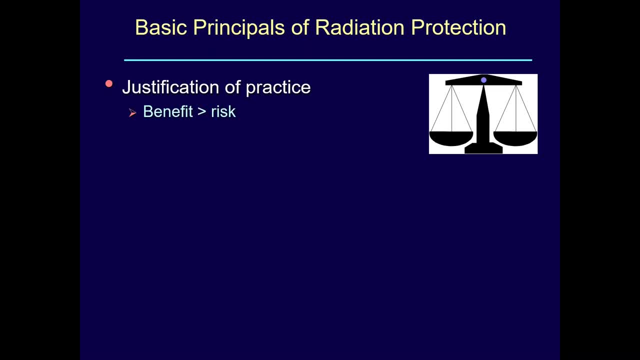 Now I am coming to the gear change, that when we say principles of radiation protection we have to first have a justification of a practice, whether the benefit is larger than the risk. if it comes to initial, you should always try to see whether an ultrasound or a MRI can be done. but we know MRI is very expensive and cannot be affordable to all. 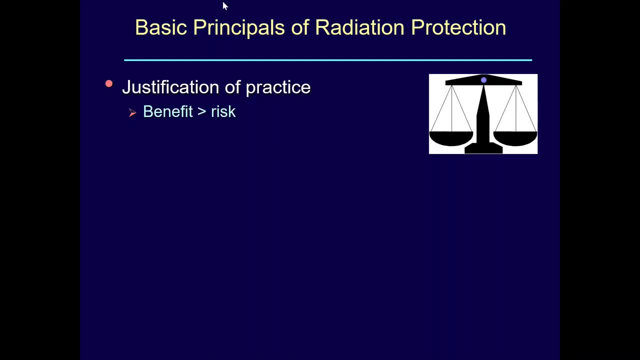 people. So you have to see, like, as I told, a chest x-ray takes very low dose and it is not at all harmful because it's just a very small dose, like 0.08 compared to 3 millisievert. So it is very safe to advise a patient even 5 times or 10 times a chest x-ray in a year. 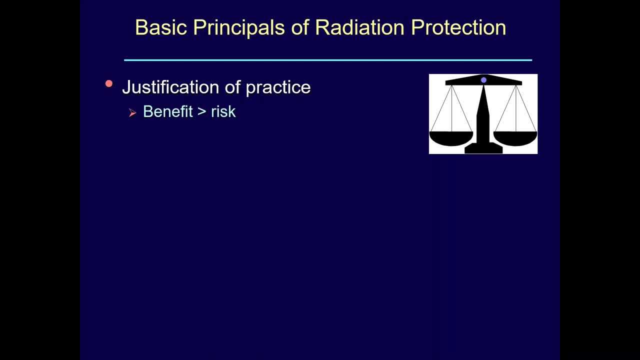 but is it true to advise the patient of a CTE chest or abdomen 10 times a year may not be, because the dose is 100 times larger. So we have to see what is the risk versus benefit. again, when it comes to female, okay, do the female population who are at the stage of giving delivery to the children in the 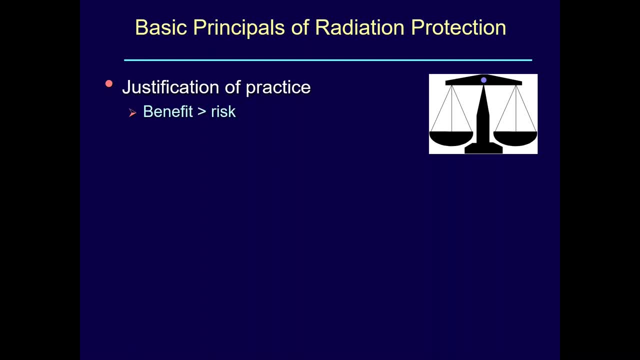 pregnancy period, do they get an x-ray done or no? they can have a chest x-ray done, but when it comes to abdomen x-ray, definitely you have to think it out. what is the benefit versus the gain? and unless until the benefit is larger, you should not go for a radiation. 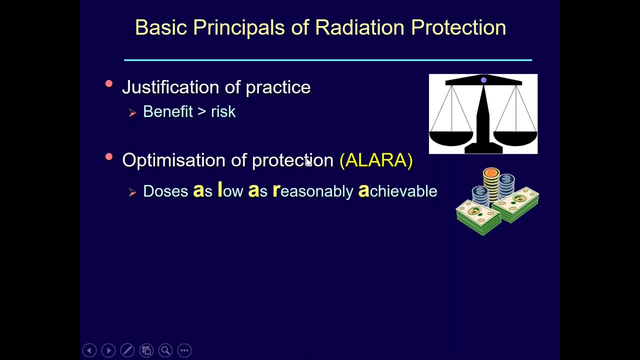 investigation. The other principle is that optimization of radiation protection is doses as low as reasonably achievable, which means if you can take a x-ray with 10 ma yes, and the image quality is good enough, you should never give ma as larger than 10 ma yes, especially for 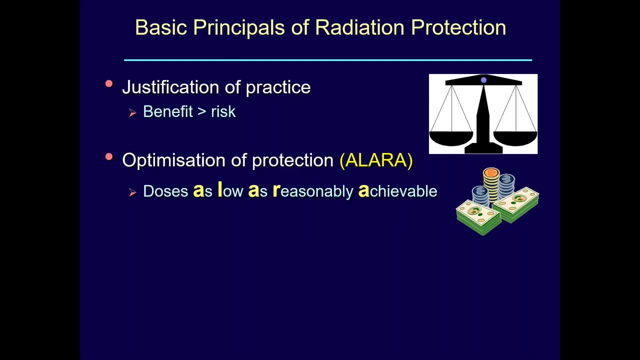 pediatric always. there is a dose care function in many of the c arms, as well as x-rays, the modern. So you reduce the dose to pediatric patients and give the least dose because you see pediatric patients are thin, they may not require the same kb and mas, so this principle is allowed. 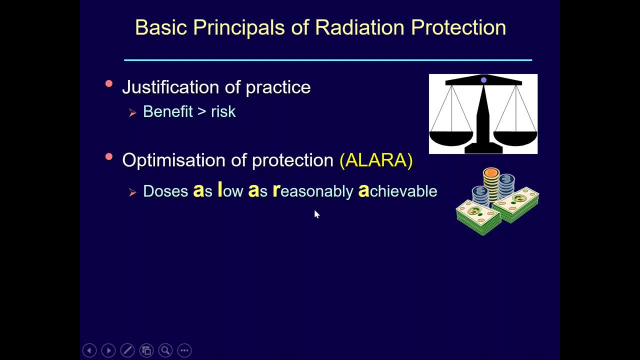 applied across in all the radiation environment doses should be as low as reasonably achievable. Then comes the other important aspect: the dose limitation, when there is a threshold dose set for cataract or for skin dose or for whole body. So this is the principle that is applied across in all the radiation environment doses should. 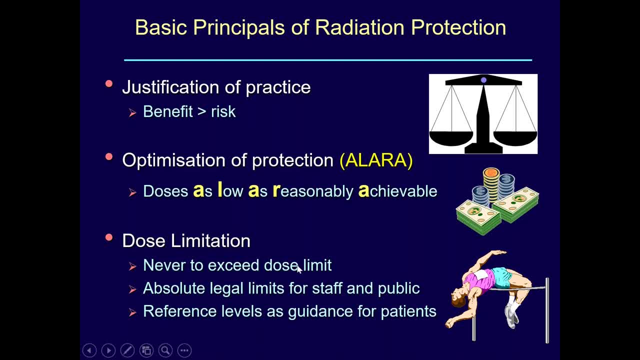 only be as low as reasonably achievable as possible. And also, if you go for st望, we do not take this movement by errors. on training versus affection development, if you go for a high ballast above risk is very not possible for your outcome or or above risk. but the wet ballast should be amobyl portable in low. 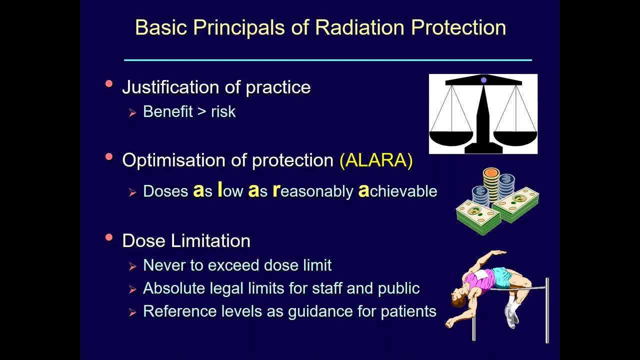 risk situations as well. that is the problem. this technique helps in this in instance of the esempio, Another study common in most rivers in the south. improve that. you know. you can have 12,13 cardinal pyod squad scene where basically 20 people to put嘛 dis dans po al. 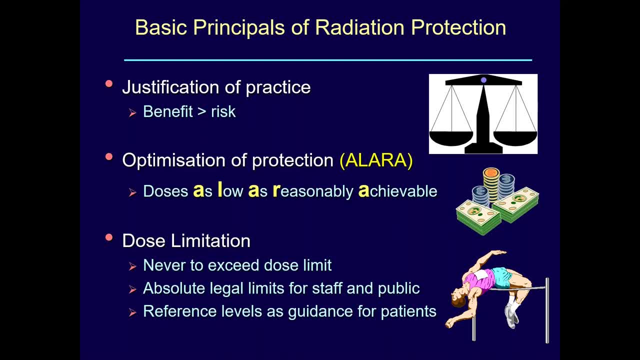 i dont put number is you're better than claire. miss college co too simple. eventually you could have been in from year there and Haus man pib- you know you tend to be put in a certain position- was especially the nursing students, the bsc students who are less than. 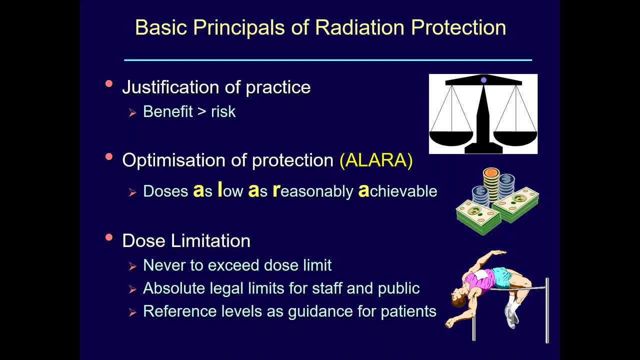 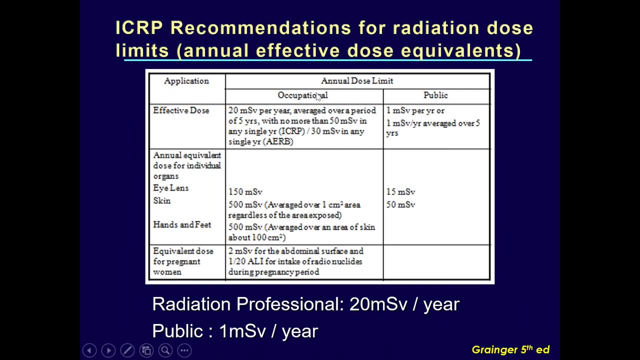 18 that those limits are much less so they have to be placed on a area when they go for practical, on a safe area for practice, and they have to be monitored if necessary. so what is the recommendation, icrp recommendation for radiation dose limits like for a annual if a radiation. how do we do this? we always give badges to radiation. 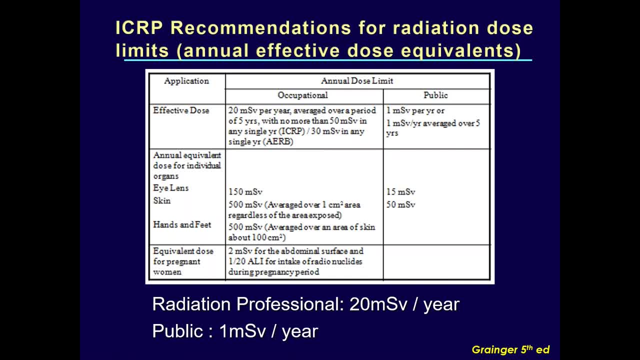 professionals, which is doctor, nurses, technician, as well as attendant and ward boys also. so different people work for different aspects. so we keep monitoring them in a radiation area, how much doses they get. if there is any one getting a larger dose, he goes for an investigation to rule out is it genuine or not genuine. if it is genuine, then there are further investigations. 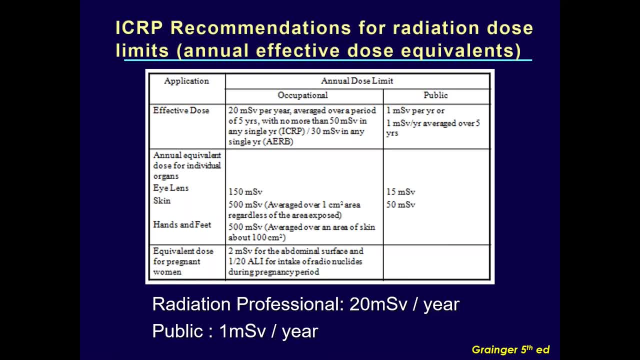 to rule out why that happened. so the radiation areas and radiation things are highly monitored for safe practice. so the atomic energy regulatory board, as well as the cp international bodies, have recommended a dose limit of 20 millisievert per year for a radiation worker, any radiation worker, and this should be averaged over a period of five years, which means 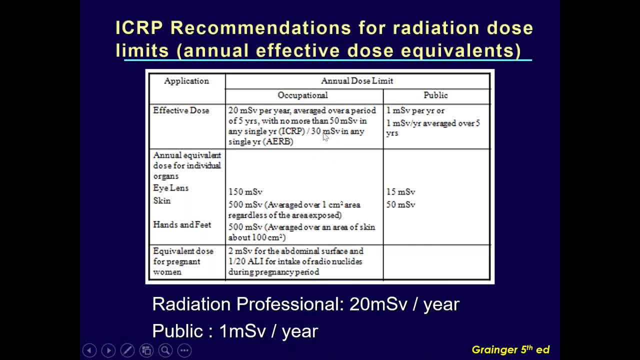 in a single year he may get 30 millisievert, but consecutively, when he is averaged over a period of five years, he should never cross over the 20 millisievert per year. okay, when it comes to public, it is 1: 20th of the occupational worker. that means the public can get only one millisievert per year. 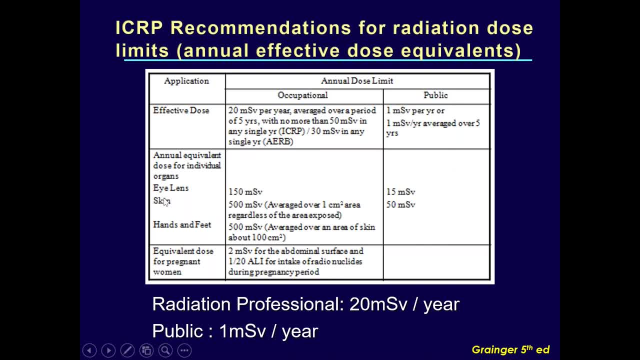 averaged over five years. when you get to the islands it is 150 millisievert, for public again 100th of it, 15 millisievert. and when we come to equivalent dose for a pregnant woman during the pregnancy period is only two millisievert for the abdominal surface region when we 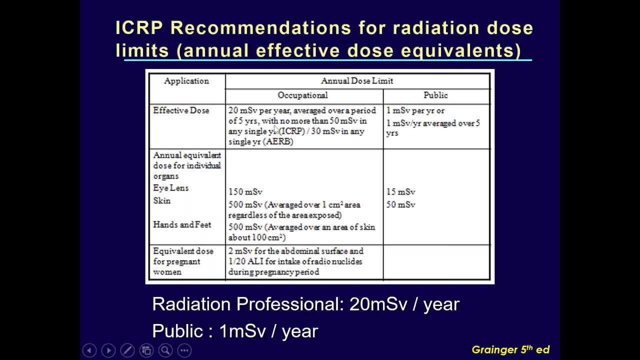 talk about whole body dose. we talk 20 millisievert on the chest for pregnant females, we talk about two millisievert for the abdominal surface. which means then, if a, pa, if a, the first trisomester is also very important and the third trisomester is also very important. so if any radiological 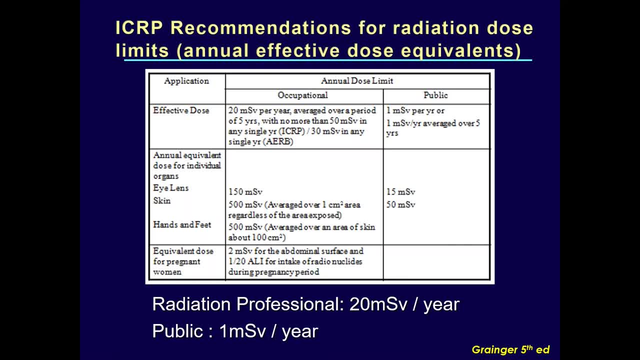 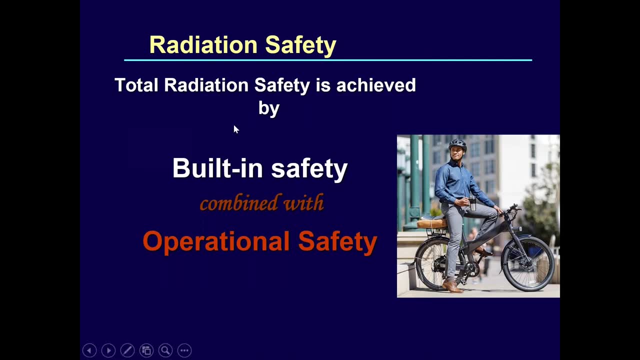 investigations have to be done. you have to consult the radiologist and take all the precaution for putting a shielding above, as well as have a dose care function to limit the radiation posible. now i'm coming to the topic of radiation safety, talking about when we talk about anything. 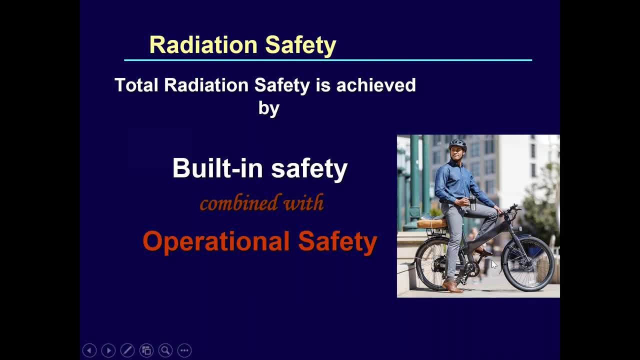 whatever we operate upon, either a bicycle or a car, always all of them have certain built-in safety. okay, built-in safety is always there in all radiation equipments as well, but we also have to concentrate on the operational safety, because if both together can only give a safe practice of befall, permitting spectrographène to perform self-explanatory splinting to the布卓 period, 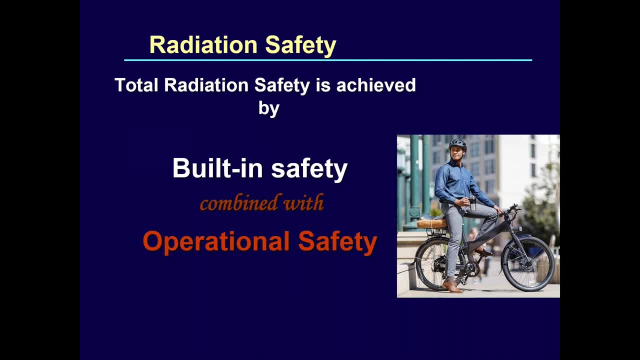 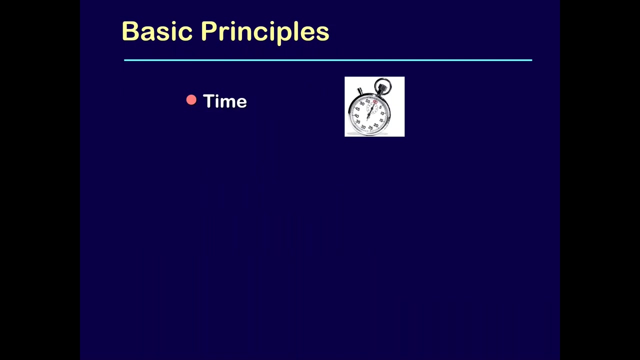 radiation in healthcare. so the equipments, all of them, come with built-in safety like a door interlock, operational interlock and all other safety features of having a protective shields, patient shields. but again operational limits and safe operational practice- sops- have to be defined for all radiation functioning. so how should we practice radiation, in all the radiation? 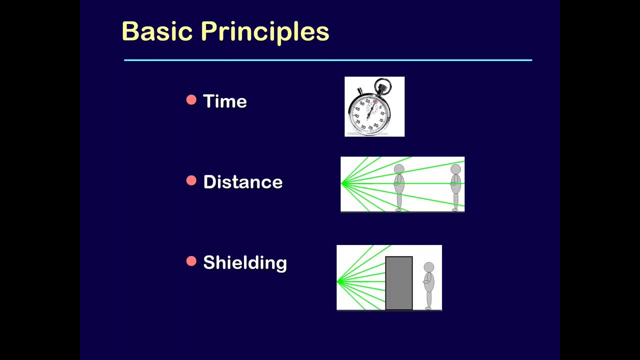 environment is that there are three important aspects: time, distance, shielding. when we come to this, is there any one thing which is most important? is the shielding most important? if we do too much of shielding, can we get away with the distance and time? it's not true. so all of them. 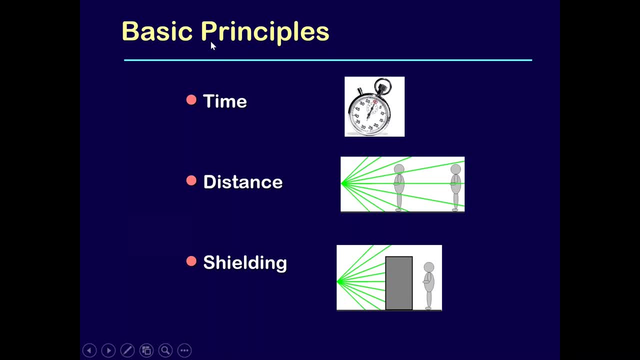 shielding, time, distance. all three are effectively needed and three have to be optimized in such a manner like, for example, if you're doing the shielding in your office, you can do shielding in your office, you can do shielding in your office, and there are many other things that you can do. 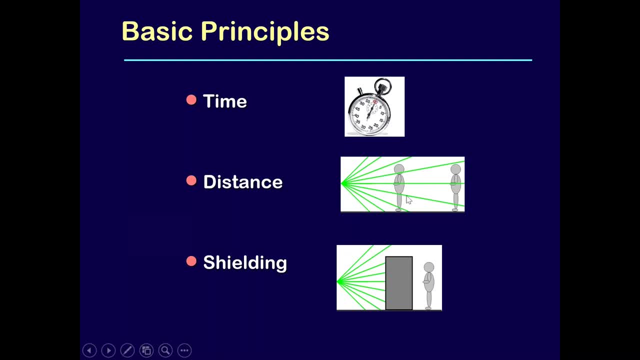 doing a fluoroscopy. I will explain it that staying one meter away will reduce the dose much. but staying one meter away you may not be able to do the functions when you are doing an interventional radiology. so there you may have to compromise the distance. the moment you compromise the distance, then you have to. 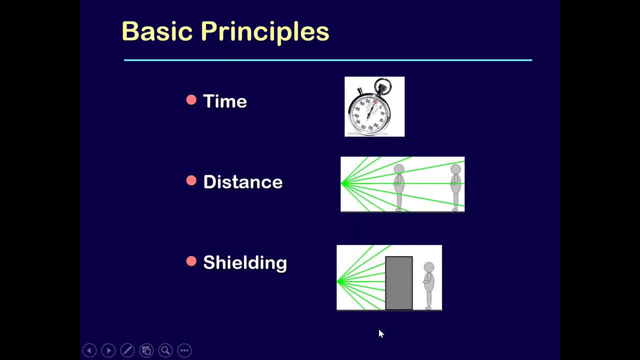 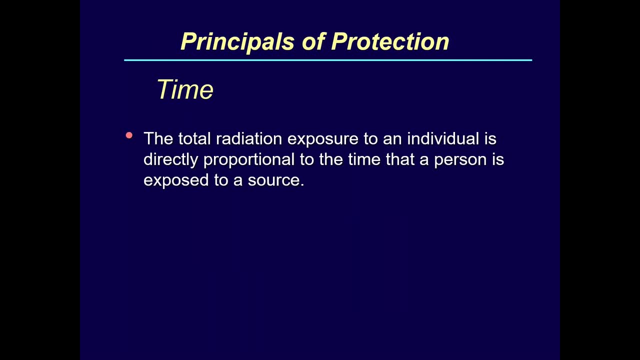 have a protective shielding material, additional shielding material inside, and try to keep the time as low as possible, so the total radiation exposure of an individual is directly proportional to the time that a person is exposed to a source, which means, before starting the beam, be well prepared. what procedure you? 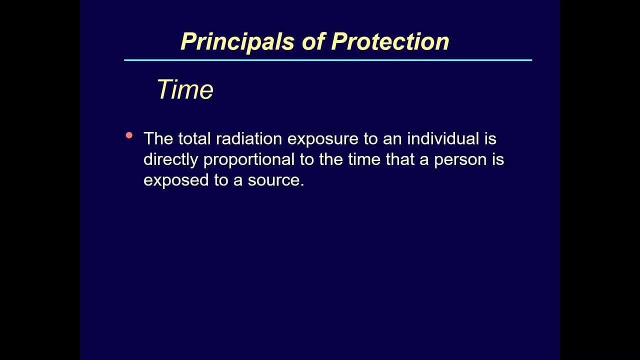 are going to do. what are the additional instruction you want to give to a supportive support staff? you first itself tell them, okay, when, at this point in time, I would be asking for this. please give me immediately and prepare for the next step. and then, when you are ready to start the next step, then you 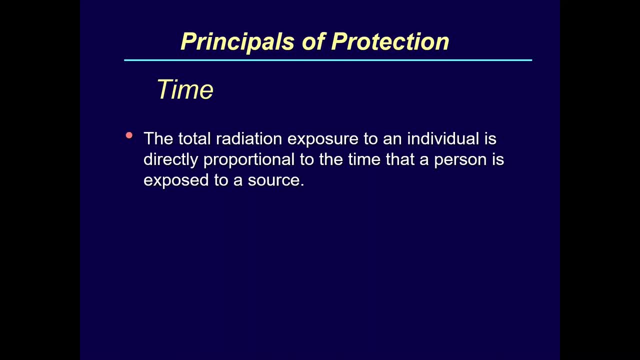 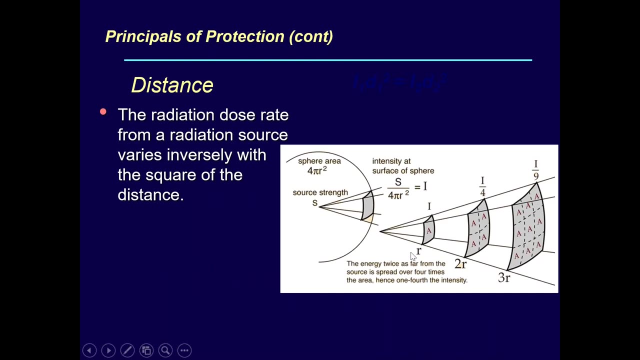 yourself for the task and then start the procedure, so that there is no time delay in the procedure for unnecessarily in between to organize something. is that okay? now the distance: distance inverse square law. if you increase the distance by a radius of one R to R, the radiation intensity falls one-fourth. if you have 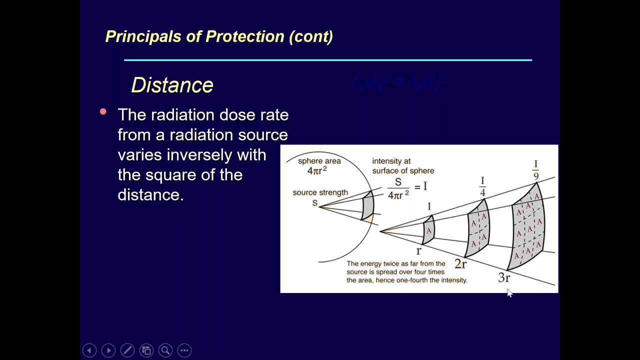 increased the distance two times. and three are: you decrease the radiation to one-ninth. so the distance you go, more the radiation inversely falls down, like the half-life. half-life also falls in the same pattern, but of course we know for certain type of a like when you are doing a x-ray. 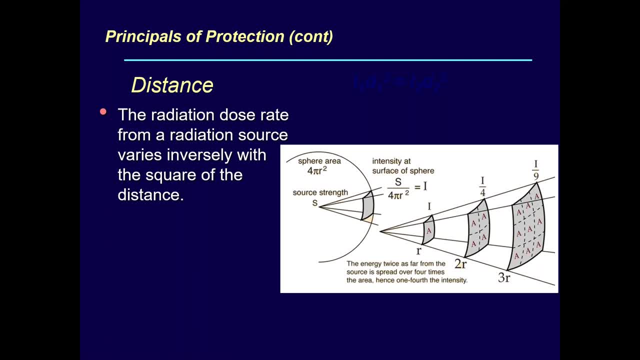 investigation. it's very comfortable ask the patient to stand near the wall, come to the control console, which is like three or four meters, and give a exposure. the staff who is giving taking a radiation abdomen or a chest x-ray is completely safe, but when it comes to intervention, you cannot do that. 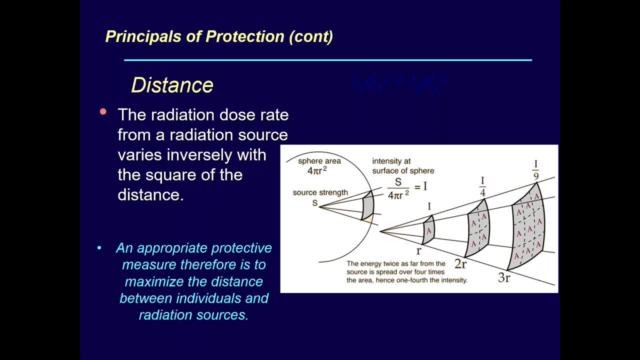 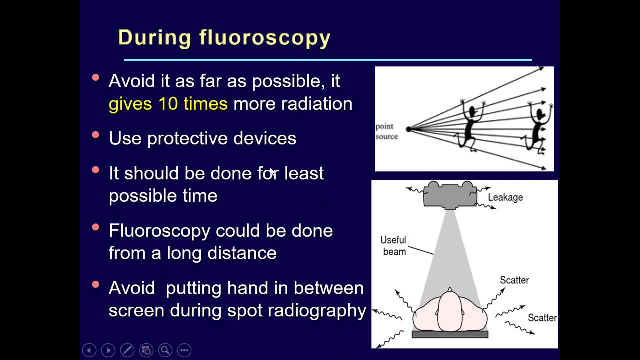 so you would be putting a led apron as an additional shielding material in order to protect yourself. that is why, when, in the fluoroscopy, you remember that you may need to use protective devices in order to additionally reduce the radiation dose to the radiation workup- another important aspect- one has to keep 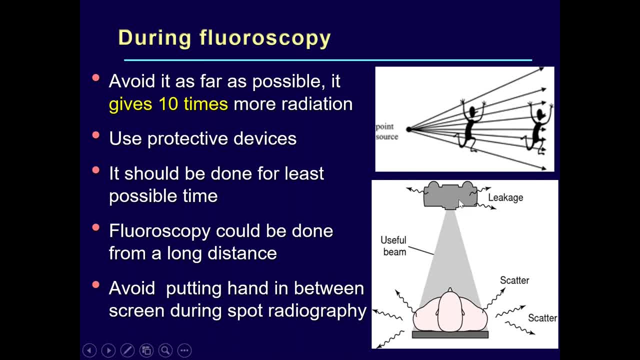 it in mind. radiation is coming from this x-ray mission and this beam is considered as a useful beam. now, what are all unuseful? the radiation which gets into the patient and scatter. this is a unwanted radiation which keeps coming. so a radiation professional, either a doctor, 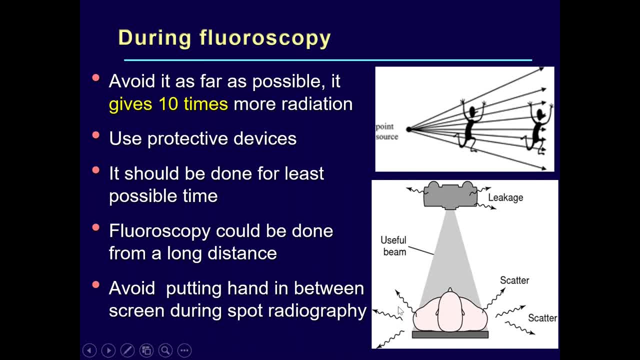 or a staff nurse who is close by will always get a radiation if they are doing an interventional procedure, so they need to wear a led apron to shield that. similarly, if a x-ray tube has gone for a servicing and the engineers didn't position the x-ray tube properly and put the 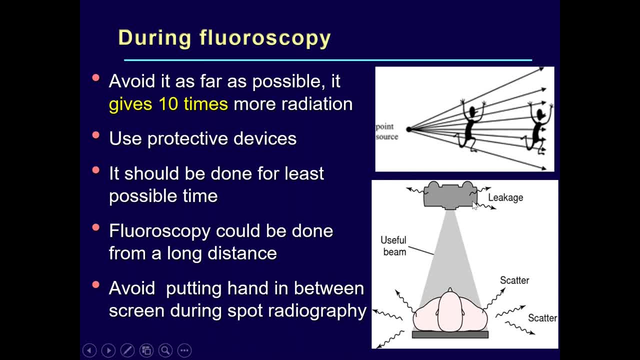 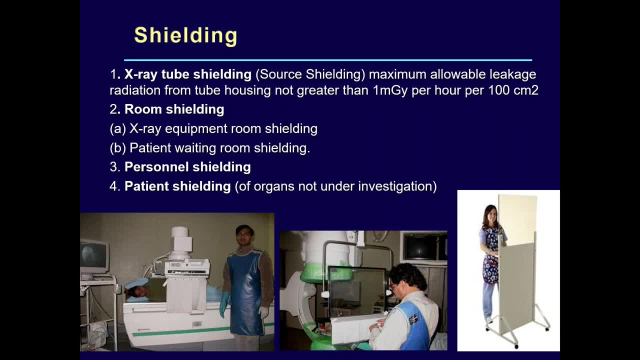 shielding tabs, there is a possibility for extra radiation leakage from the apparatus of the source housing. so a complete quality assurance and quality control of the x-ray equipment after every repair is mandatory. so here in this you could see that this x-ray tube, x-ray c arm, where you are doing a. 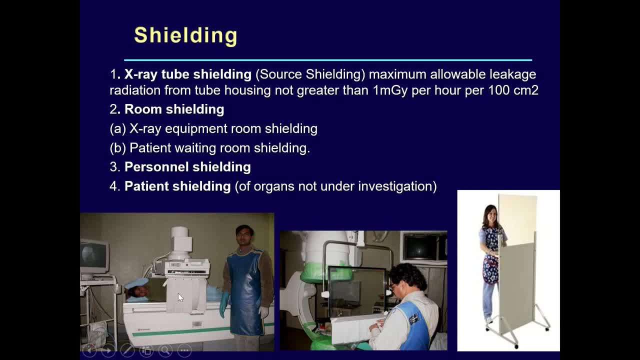 fluoroscopy that was physically radiated. in this case you would be talking to the local health department about your x-ray tube rosse 膨 drag to see if there is something can happen in this body and the unclear, and then the x-ray tube with that Stuff börjar. 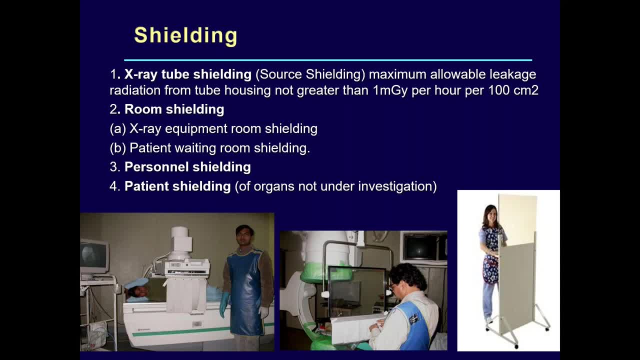 the animal weight does, and we further. it has added two points, and these two points are combination. looks so clearly, though. you see, the on standing side of the Île is X-ray tube wall, Feuerlu, and the patient is walking, walking. this is the station is. 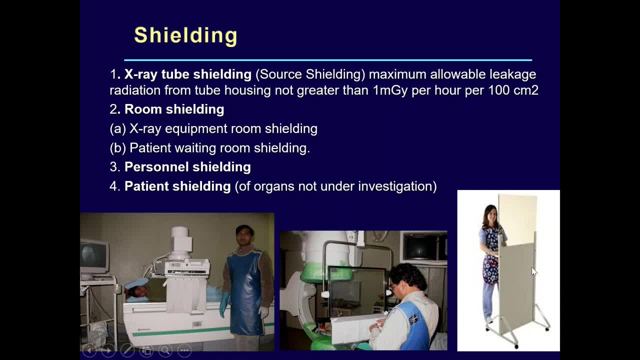 underile of the donase. have US discussable ionized? we can see all the different ways. fn okay. similarly, you have bedside trolley with a lead glass. have you heard about a lead glass? we always see a glass which you can see through, but there are lead which is mixed in this glass. 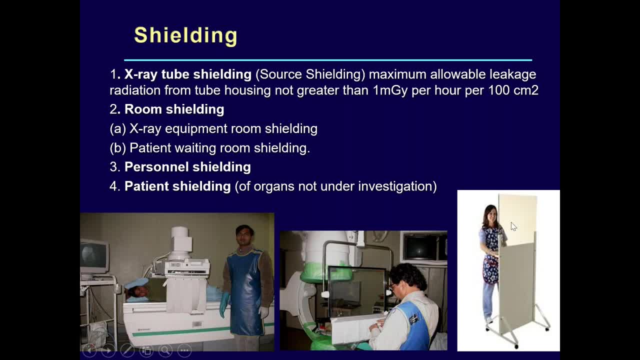 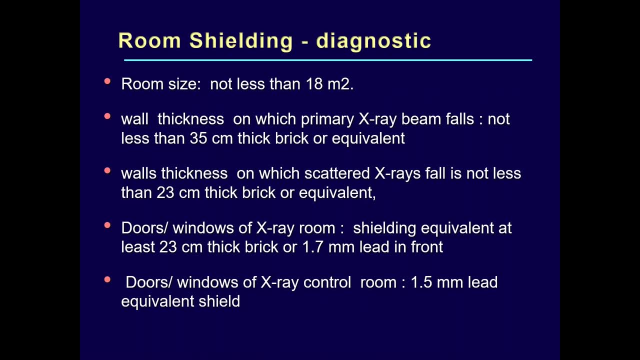 and it can attenuate like a shielding material. so in fluoroscopies we have a lead shield with a lead glass. now for a ideal x-ray unit, the room size should be at least 18 meters and the wall should be made of brick 35 millimeters and there should not be any windows where the radiation can. 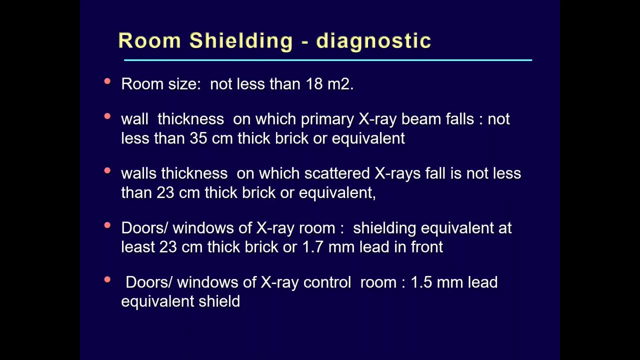 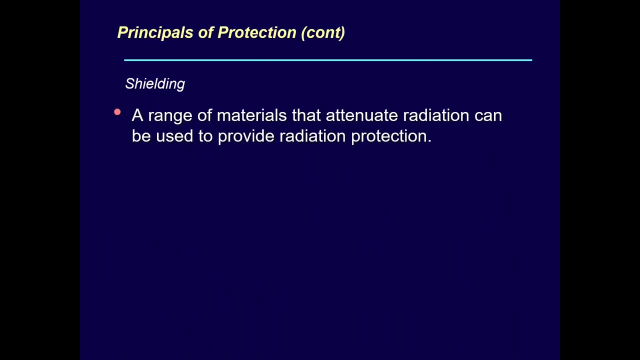 scatter and someone can sitting adjacent to the x-ray installation gets the radiation dose plus. the lead doors and the windows are always lead lined. they are 1.7 millimeter lead lined on the door for all x-ray installations. now coming to the shielding, if you come to the 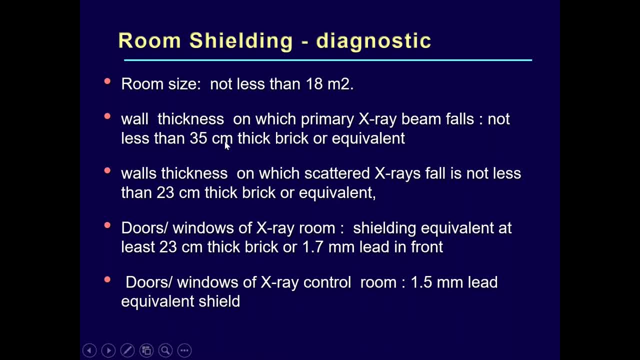 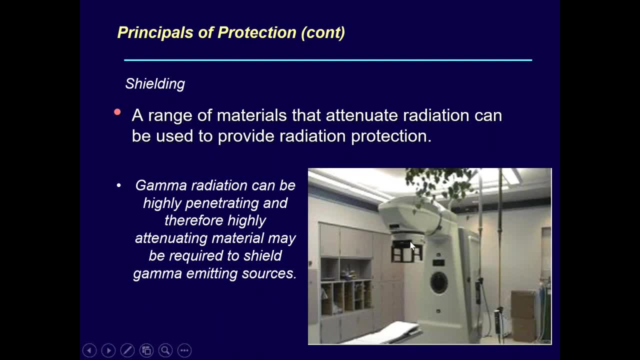 shielding for a x-ray installation is only a brick wall, but when it comes to nuclear medicine- pet pet, gamma camera or radio therapy, tele cobalt or a linear accelerator, the shielding is very large because they use a very large radioactive isotope of a very high strength. okay, so where these kind of a units can? 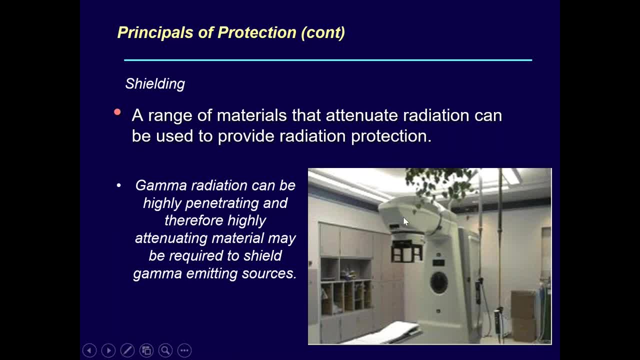 the source is generally kept here and the source is house housed on a uranium container which is much more shielded and safe for practicing. this rotates across. the patient is lying on the couch and this can be shifted up and down and the couch rotates across the patient, I guess. 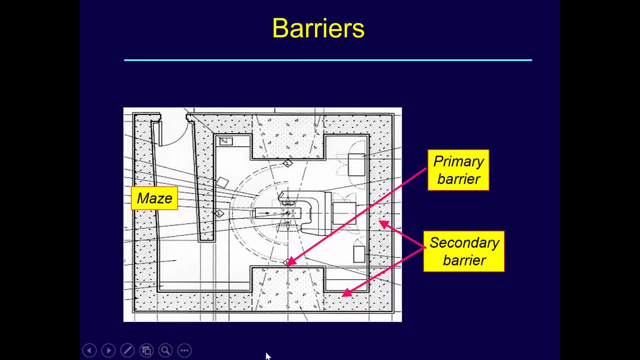 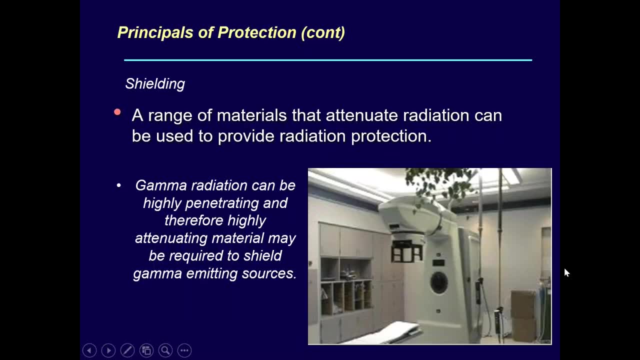 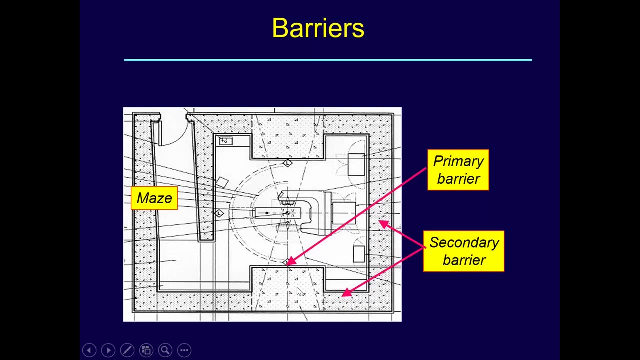 axial CT and you can treat the patient, so the shielding requirements are very stringent. this is: this is a cross cut, like this: I'm doing two cross cuts, one this and one sagittal. this is a cross cut showing the maze wall, the person when you enter, like this: 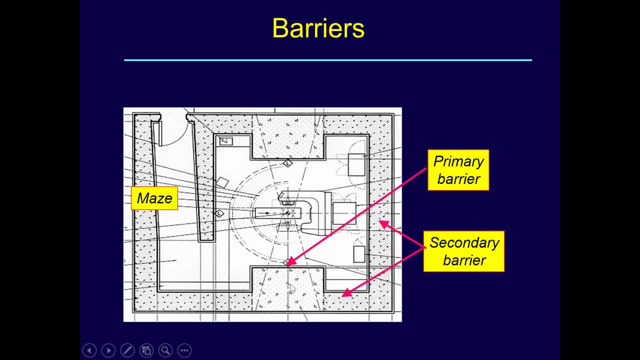 the radius of the wall is shown. the equipment is a house here. the primary radiation beams falls here, so you see the shielding thickness of this. this can be around 1.2 meter to 1.5 meters, or even 2 meters. for a high-energy mission, these are around less than 1 meter, so 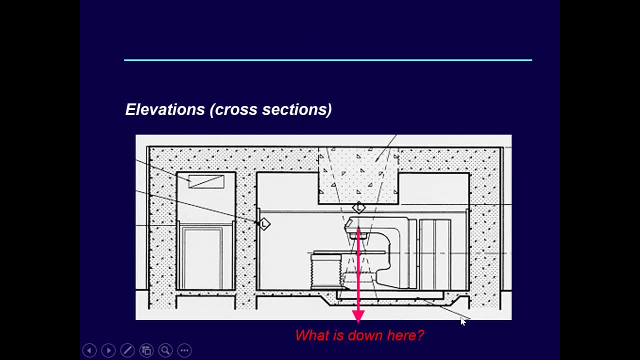 these maze walls, a huge construction is very well needed for the purpose of ice shielding, which we call it as a primary barrier and a secondary barrier. and if we look into the sagittal view, below is the floor and this is the fall ceiling, like in our department radiotherapy. above the radiotherapy is our mini auditorium. so 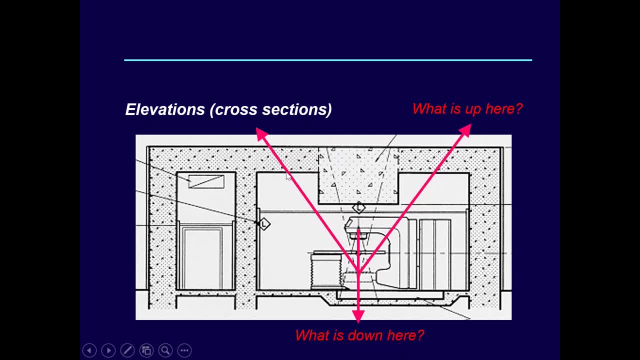 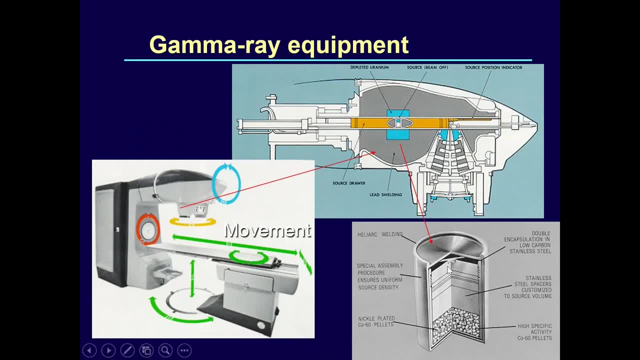 the barrier. if you see the beam primary barrier, which is of a huge concrete thickness right like two meters, compared to this is one meter. so a heavy construction is required for radiotherapy purposes because this gets a cobalt pellet which gets into BRC for artificial radio isoto bombarded from a neutron cobalt 60s. 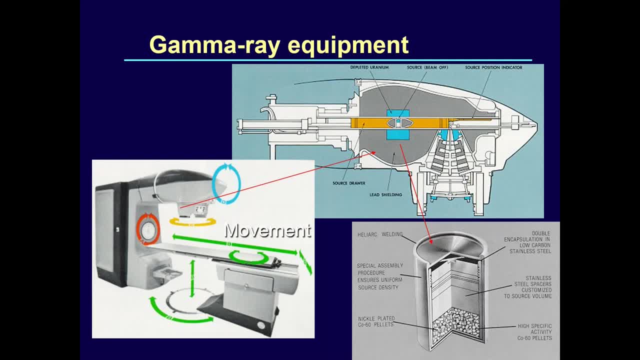 cobalt bombarded with the neutron to become radioactivity and it decays to nickel, emitting gamma and beta rays. so this radioactive source is housed here with the thick container of tank tungsten with uranium mixture and this source due the pressure mechanism pushed here for source on. 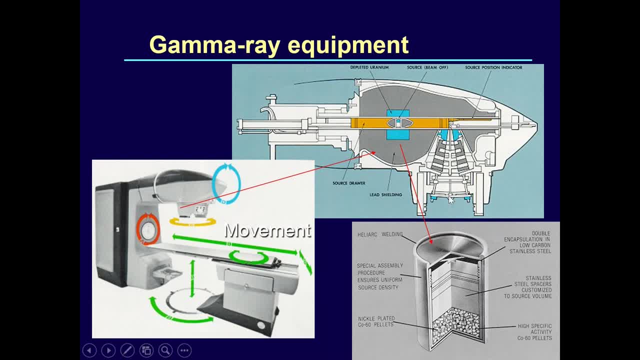 and off position when it comes here. the beam is treated here for the radiation, so there could be a possibility of a radiation source truck and many other incidents where people have to practice this very safely. i'm not going to bother about you with the entire radiotherapy practice. so coming to what? 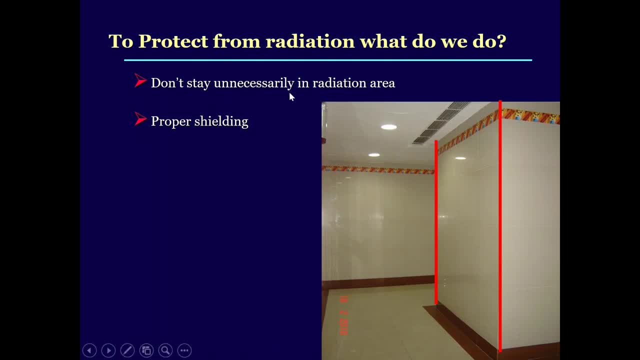 kind of a practice we need. so don't stay unnecessarily in radiation area, which means i'm not asking you. please don't do not come to radiotherapy. okay, you are safe to come to radiotherapy and even once in a while you can go into a radiotherapy installation and see. 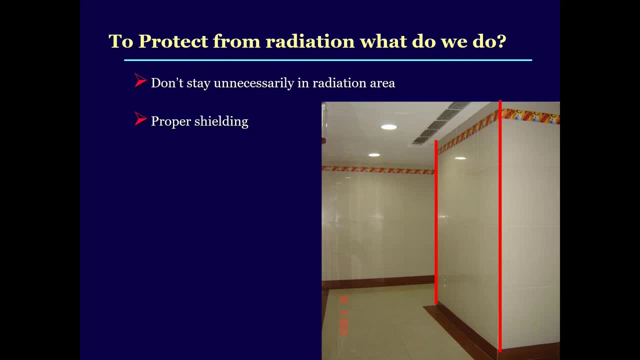 but i know a lot of anesthetists do- posted on the radiotherapy equipment for sedation of the children during the radiotherapy procedures. so they come frequently but they cannot be posted completely. if they're posted completely we have to give them a lot of time to do that. so 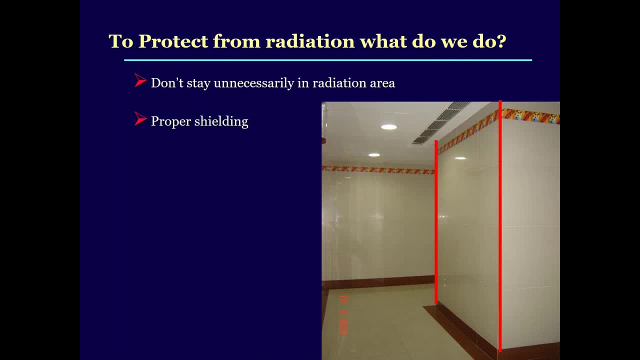 we can give them film badges and monitor the radiation doses. these are the regulatory requirements, otherwise radiation may even the control console. the radiation workers are as safe as the other population like. i would like to tell you we are monitoring the radiation safety for the all the radiation workers. we don't see. we see a small increase of one millisievert extra for the. 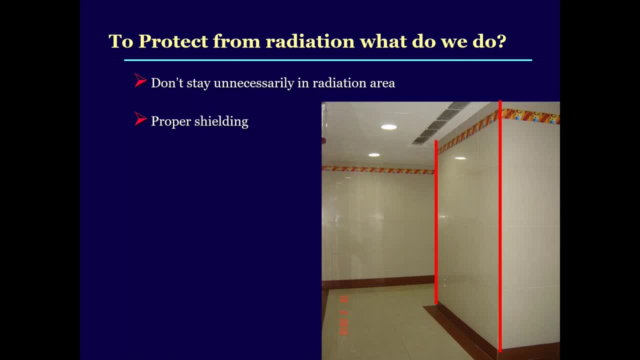 radiotherapy department or a nuclear medicine department. sometimes nuclear medicine is slightly larger than radiotherapy or radio diagnosis because they deal with contaminated radiations. although the radioisotope is of a small activity due to contamination process, sometimes they get a radiation and even then the radiation is, i would 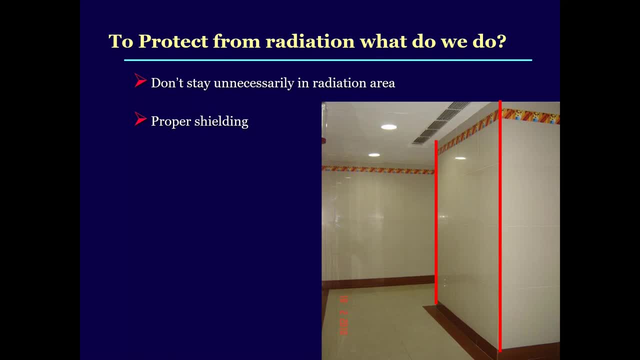 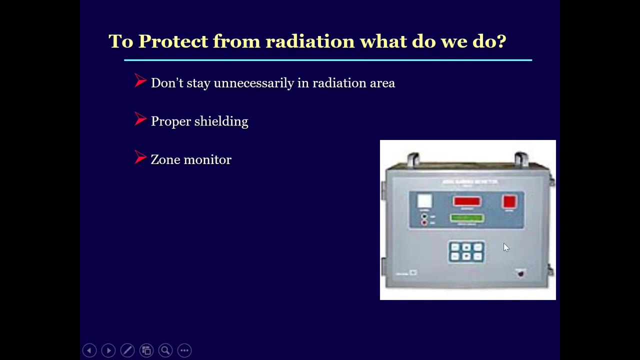 say, half of the background radiation on average. i don't see that they cross beyond 1.5 millisievert per year, any radiation worker in this institute, okay, so for this installation you may be seeing zone monitors which are monitored to say that the radiation is not being transmitted to the radiation. 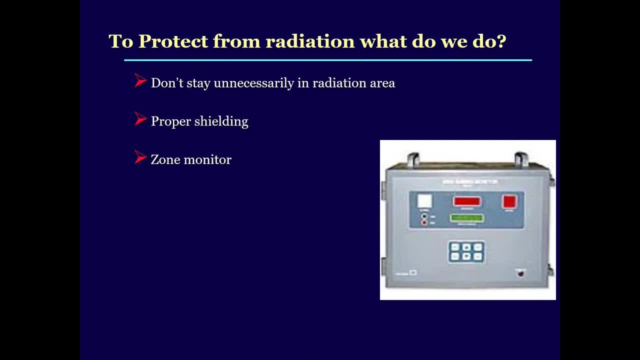 department, but this is the radiation sensor which is used to determine whether the radiation is safe or not. so when red, when you are entering a radiation department, you should see whether there is a survey meter, and the survey meter is showing a half position. if it is off, it is safe to enter. 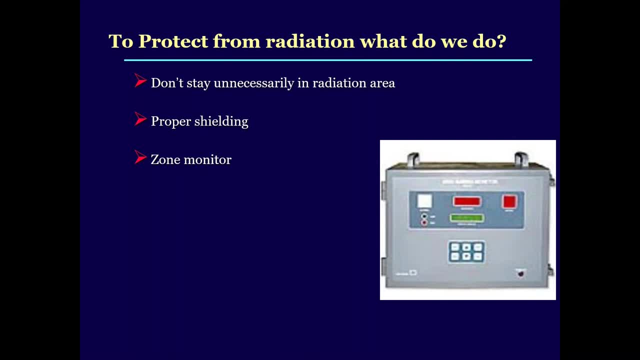 in. if it is not, it is not safe to enter it. so this is for general public and for radiation fraternity as well as medical fraternity, to understand and adhere, to respect all the monitor and door interlocks and other things and see these symbols when it is x-rays on. 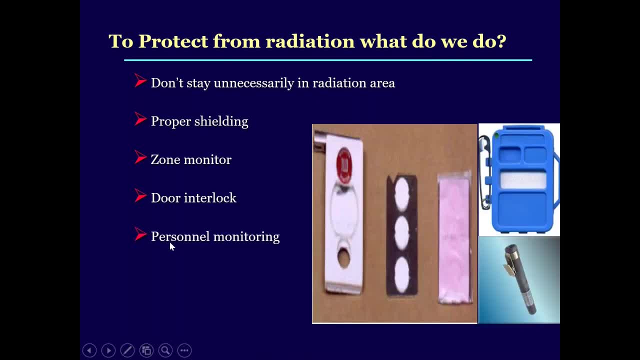 interlock showing that the radiation is on. so now, apart from this area monitoring, you have personal monitoring devices like the TLD. the TLD is a thermoluminescence dosimeter. there is a lithium fluoride capsules. three capsules are kept here and this is bad on the badge, like the chest for the radiation. 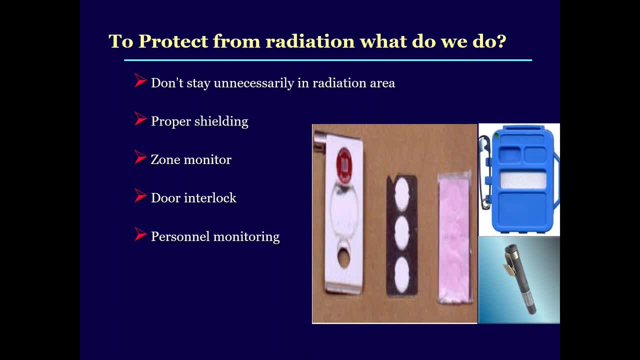 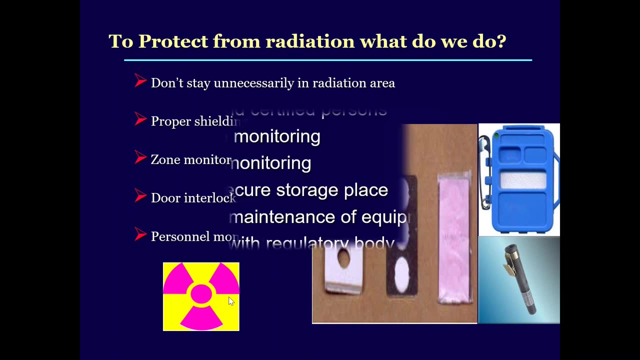 workers to know what is the radiation documented on them by working in this radiation environment. okay, and for all radiation environment, you will be seeing radiation symbols like this, and I will tell the specific definition and the dimension of the symbol in the last slide. so now coming to operational. 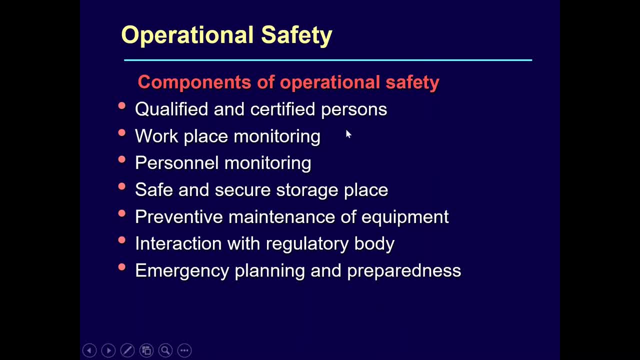 safety. radiation equipments cannot be operated without certified or trained persons and all radiation installations have to be monitored every monthly for radiation safe survey and personal monitoring by personal film badge services and all the radioactive source has to be securely stored and inventory to be maintained, and there has to be a emergency preparedness plan in case of a. 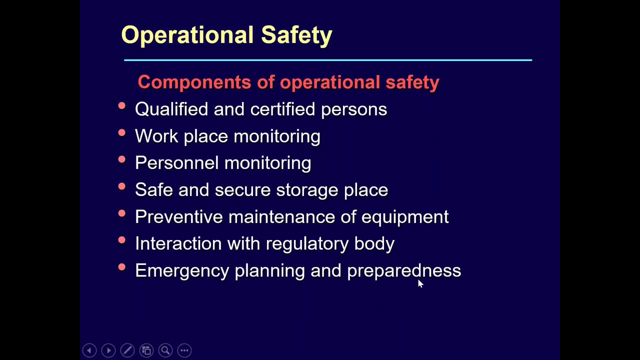 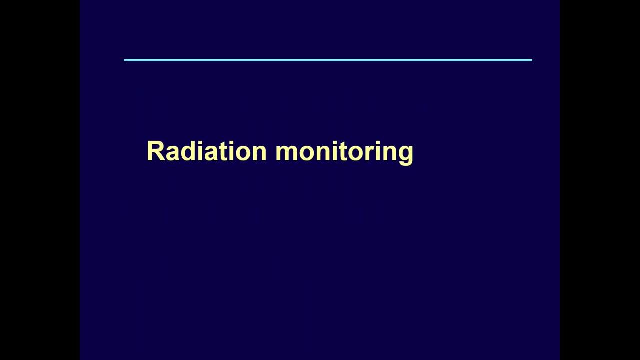 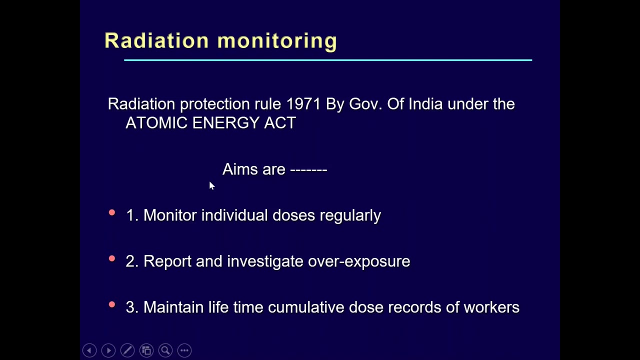 radiation accident in radiotherapy or nuclear medicine, in radio diagnosis? always there is not. a major accident can happen, but still all the equipment has to be monitored for leakage radiation and scatter radiation on a periodic intervals. so when you talk coming about radiation monitoring, monitor individual doses regularly of a patient, of a staff every three months. the staff is mean. 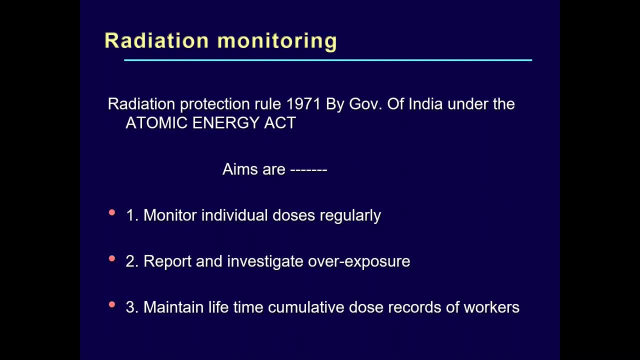 say, given a new badge and the old badge goes to a respiratory research laboratory and they read the personal monitoring doses and share with us. and these reports are available for all radiation workers. and this radiation worker records are lifelong. it is a cumulative exposure for their life. so 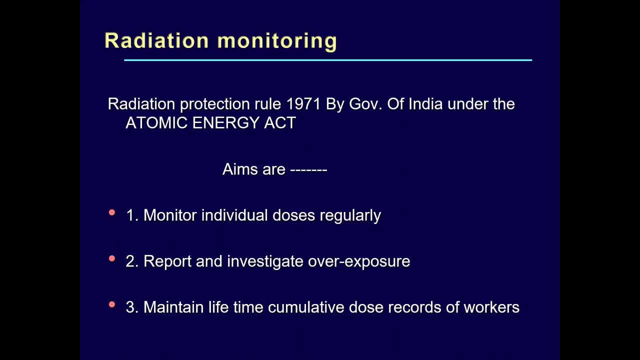 whenever they go from one organization to another organization, they have to disclose their personal monitoring film badge number and the personal monitoring institution number for them to add their radiation exposure for their cumulative exposure. it is a very important regulation by the Atomic Energy Regulatory Board that you cannot hide your radiation dose, what you worked. 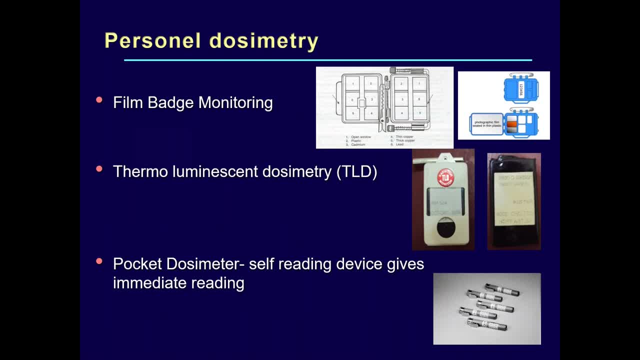 in any organization. so there are various types of personal dosimeters, like a film badge, thermoluminescent dosimeters and, as these thermoluminescent dosimeters remain a critical part of their encoding over time and they confirm on non, versus a secondary dosimeter every 10 years, 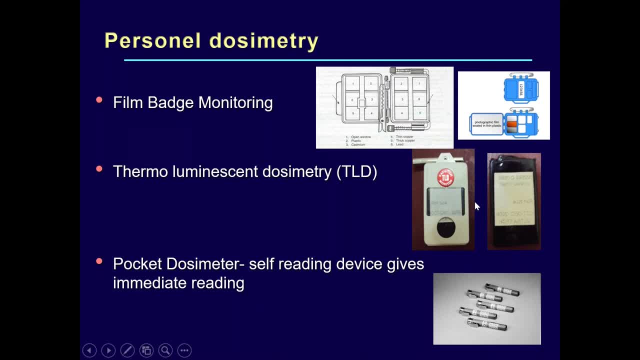 and dosimeters we can assess only after three months because a radiation accident we cannot know immediately. so for that purpose we have pocket dosimeters and bleepers which will give bleeps depending upon the intensity of radiation. so these kind of radiation instruments are used by the radiologist, nuclear medicine specialist technologist and the radiation 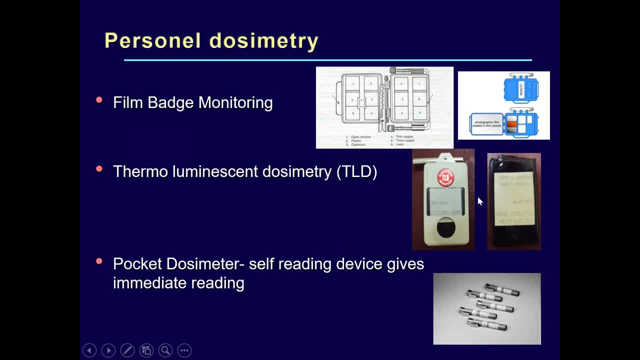 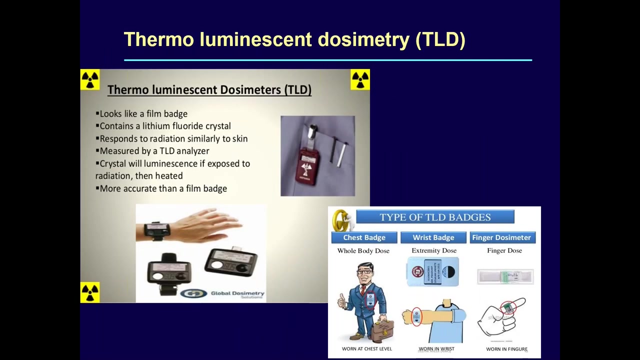 safety officer to handle radiation emergencies. and these personal monitoring tld badges are wired by every radiation workers and if you are posted in radiation work area doing c arm intervention, you should demand for a film badge and you should wear it routinely whenever you are in the radiation area. and apart from the chest x-ray, you could also find the nuclear 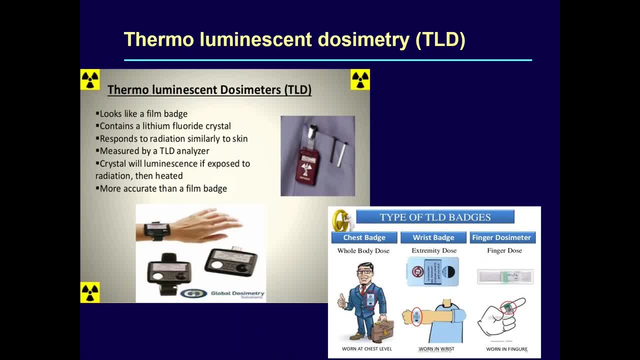 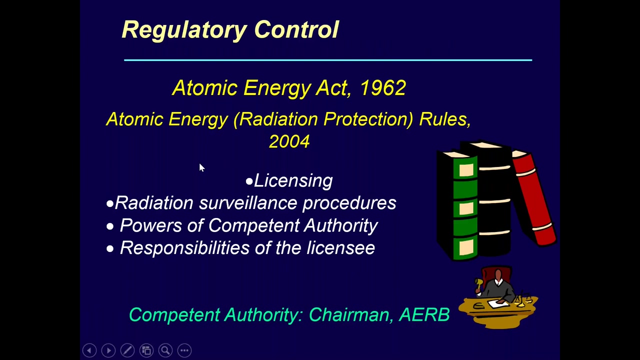 medicine. people keep wearing some wrist and finger also because if they do so much of exposures by hand during a Invalidation- Invalidation We are auto Invalidation Invalidation- competent authority of Atomic Energy Regulatory Board. And if you don't do all these stages, 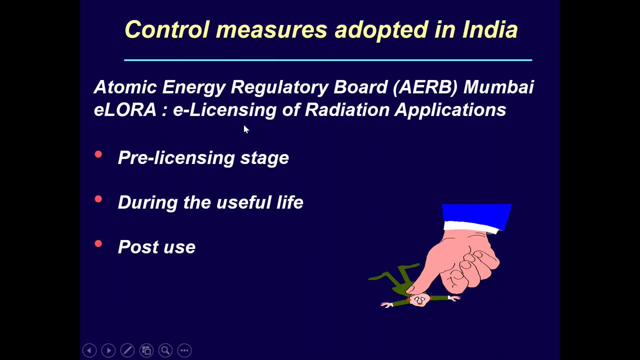 and anything anywhere harmful. they have also now started e-licensing of radiation applications, which they call it ELORA. That means all radiation equipment. when you procure, you have to disclose them and you have to take licenses. When you decommission, you have to tell them all the. 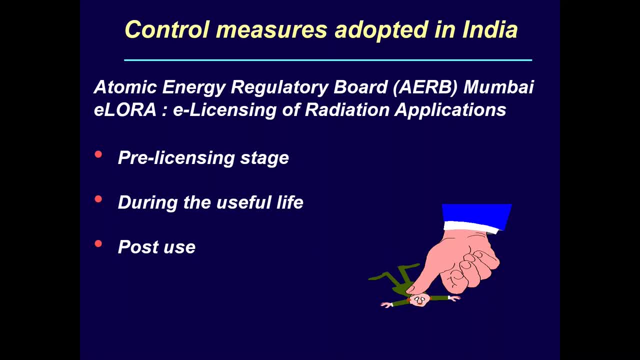 decommissioning processes and dispose it off. A safe disposal is also very important And all radiation workers have to be enrolled into the ELORA And they do surprise checks and they do come for visits to have an emergency survey and emergency visit And if they find, 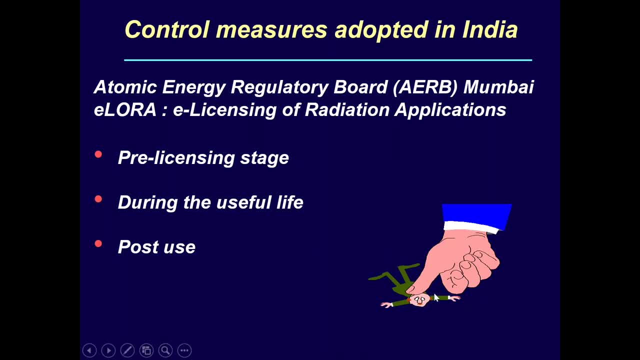 anything, they can penalize the institute and they can put a full stop to the entire radiotherapy or radiological or nuclear medicine services. to stop till the things are in order. So what are the prerequisites for licenses? We have to have any equipment before procuring. 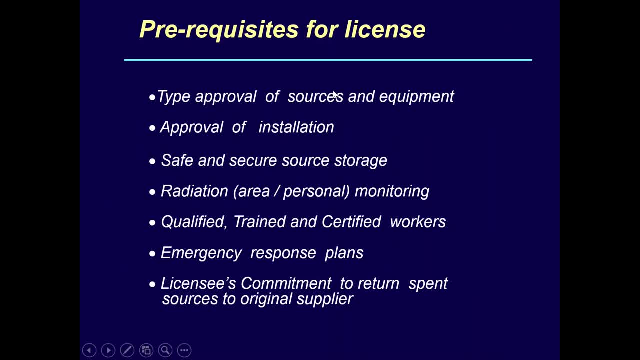 the equipment. You have to tell what type of equipment. You cannot just pick any radioisotope equipment anywhere. Those equipment have to be type approved by AARP And you have to approve the installation. You have to disclose the storage pattern. You have to confirm the facilities for the area and personal monitoring. That means a. 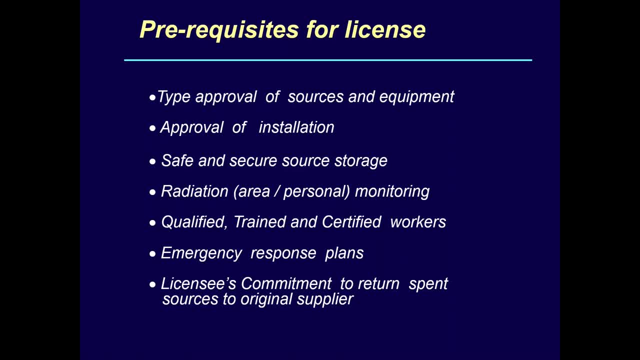 new institution If you are creating, if you have not applied for TLD services and the survey meters, they will never give you a permission to start even the X-ray And similarly, you have to check all the information. We have to have clear state databases. do all the. 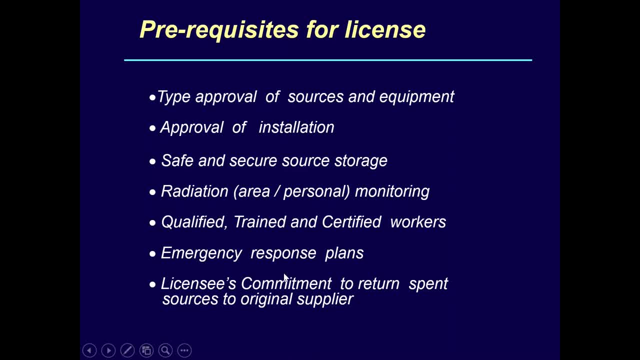 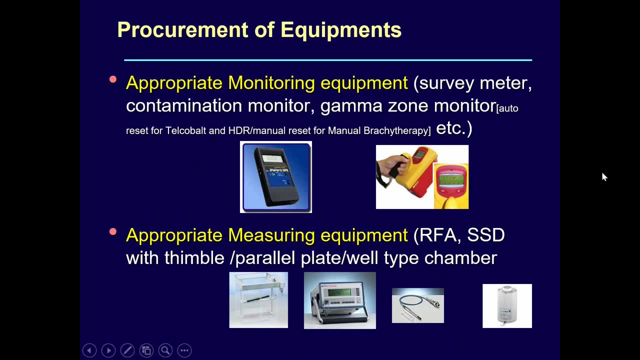 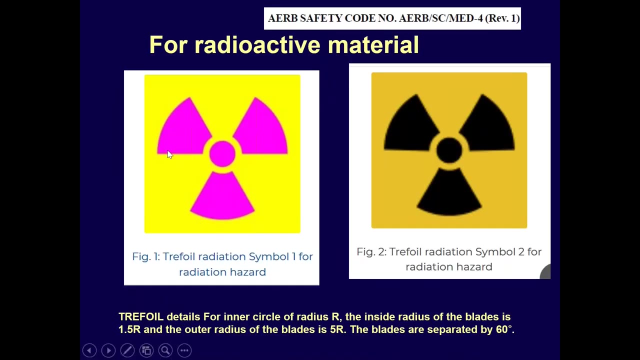 you have to have qualified staff and enrolled into the processes in order to have the licenses up and ongoing. so, as I said, there are various instruments used for surveying purposes and for those measurement purposes, in the CT and in the linear accelerators, which I will not go on deep, okay, so the last one I want. 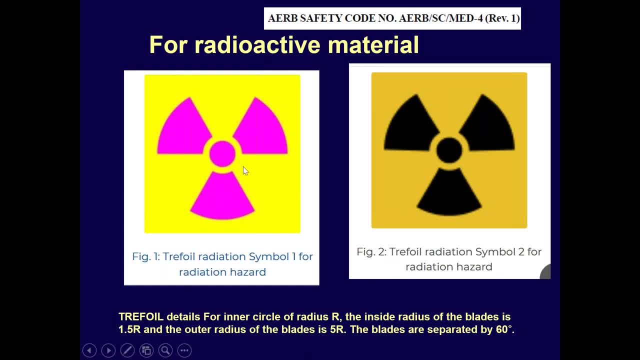 to say, the radioactive isotope symbol should be either of the either of these two, figure one or figure two. it could be either a magenta color or a black color and you could see a small circle of radius R and if this is, are one point five times should be these blades and one, four and five times will be the. 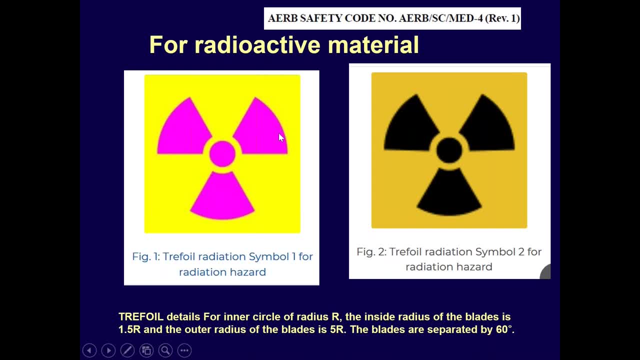 outer ring. the dimension and the ratios are important. you cannot just to draw something and put: this is my radiation symbol. you have to have the radiation symbol idea to the principles and the regulations regulated by them. now, if you have a radiation symbol, you can draw a small circle and put it in this. 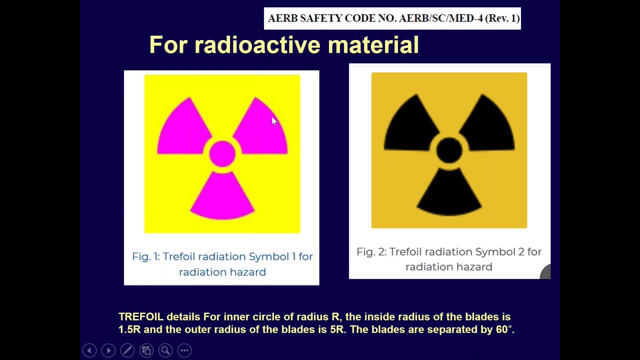 and it should be exactly in this dimension. and these blades are 60 degree. so 60, 60, 60. you see three blades and three vacuum space together form 360 degree, so the angles and other things have to be respected in the same way. so this is what is the ideal radiation symbol, which you should be. 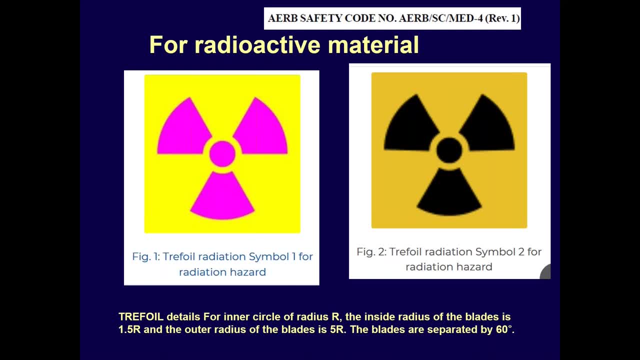 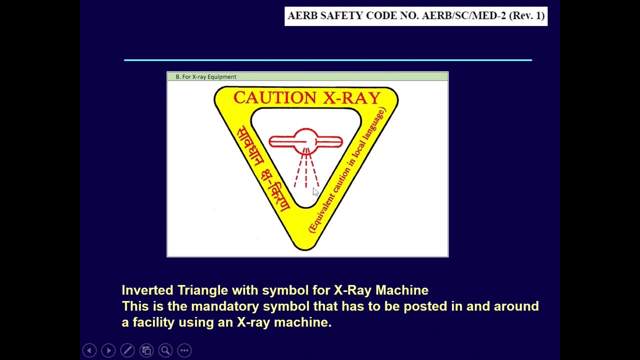 able to see in radio nuclear medicine department or radiotherapy, or even in endocrinology and many other immunology, where you use research for radioisotopes and wherever you have x-ray installations. the x-ray installation symbol is this x-ray coming out by this and there should. 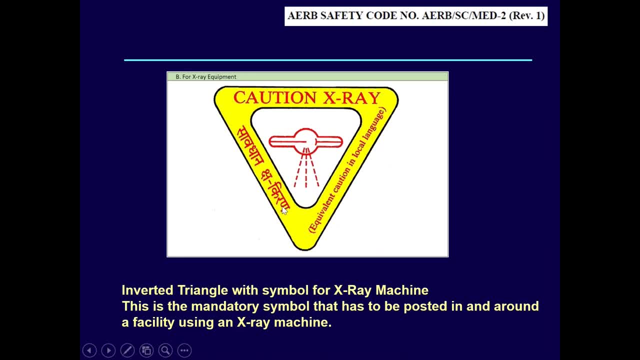 be a caution x-ray in english and you have to write this and it also to be written on hindi like this. so this is the regulatory requirements: wherever there is a x-ray installation, this symbol should be placed, and in the ct and other thing also, we have to put a symbol like this for pregnant.